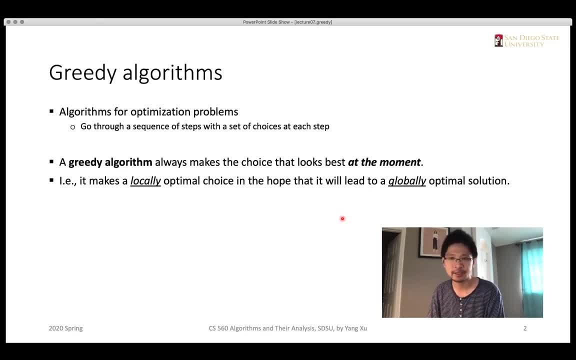 access to all the information needed, or global information needed, in order to solve the problem in a guarantee, to excuse me, to get the guaranteed global optimal solution. but instead we need to step back and to look at what the local optimal solution is and to and we simply choose that local optimal solution in the hope to. 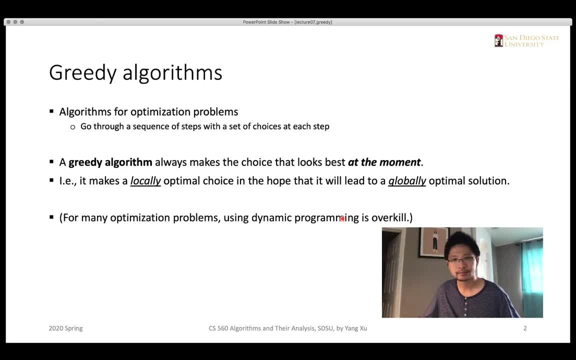 obtain the globally optimal one, and this type of algorithms has a very close connections to the dynamic programming algorithms that we have been talking about so far. but for many of the optimal, optimal optimization problems they can be solved by a dynamic programming algorithm. but sometimes using dynamic programming is. 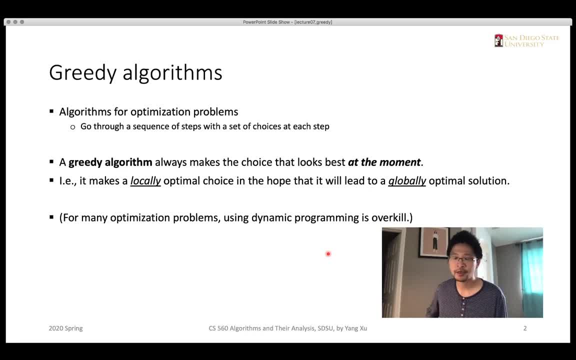 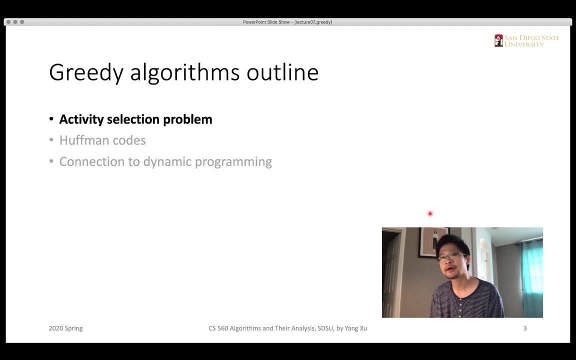 an overkill, it's unnecessary to solve all the solve problems. ok so on. compared with DP, greedy algorithm usually saves, saves more time, saves more energy and and also leads to global solutions, the optimal solutions. so in this lecture we will have three topics. we all in this lecture, in this video, we all talk about this. 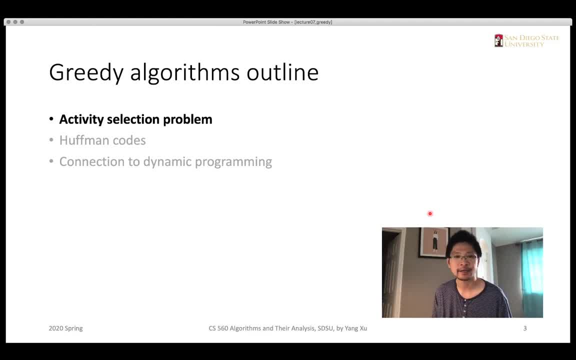 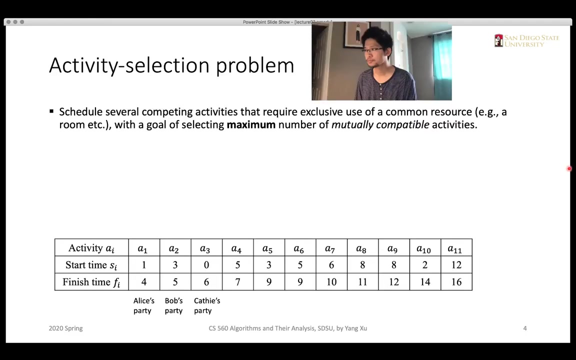 particular type of question, which is called activity selection problem, and this is a very typical problem that can be solved by a greedy algorithm, and then we will talk about Huffman codes and the general connection from really algorithms to dynamic programming within the next video lecture. so the activity selection. 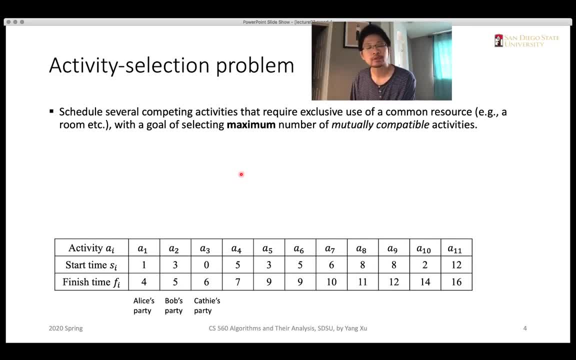 problem is to schedule several competing activities that require exclusive use of a common resource, so, for example, a room, and the goal is to select the maximum number of activities that are mutually compatible. okay, so, for example, given this table of all possible activity activities to be scheduled, not all of them are compatible. 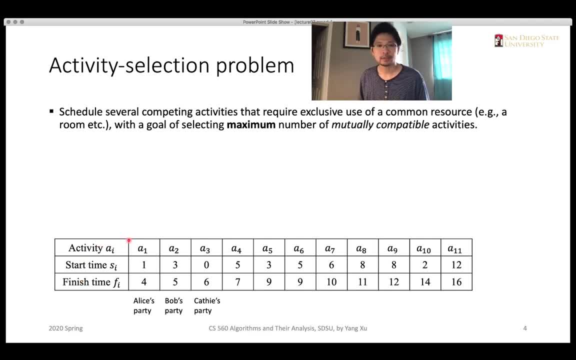 with each other. so look at the, for example, the activity one. it starts from 1 o'clock and finishes at 4 o'clock. say, it's Alice's party. so it is not compatible with the second activity, activity 2, which starts from 3 o'clock and by the time it starts the. 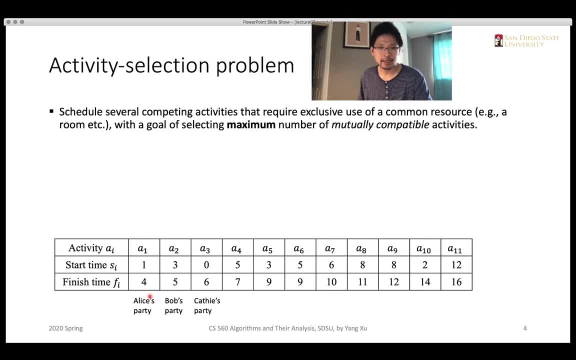 first, the a1 at Alice's party is not ended yet. okay so, these two activities, a1 and a2, they cannot be selected or scheduled at the same time. okay so, because we are scheduling the activities for one room, for a, a hall home, and we cannot let a1a2 happen at the same place, at the same Hall, at the same time you. 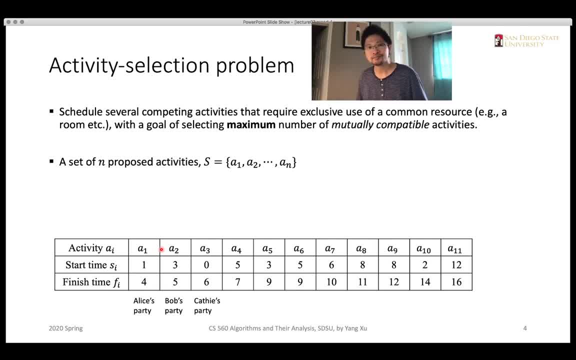 time. okay, so we are given this information so for for to solve this problem. we're given this information from a1 to a- n and in this case, we have 11 activities possible, and our goal is to select a limited number of activities that can happen in the same place. okay. 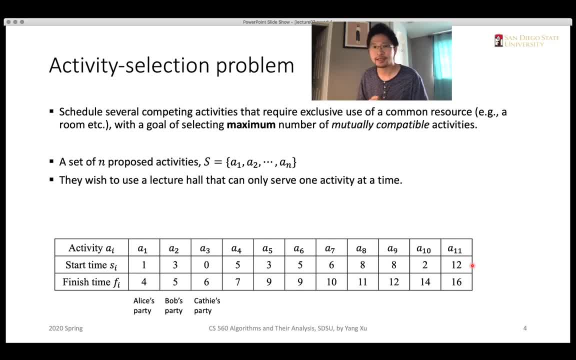 and we wish to use one lecture home and we wish to use one lecture hall that can only serve one activity at a time, and but the goal is to select the maximum number of activities because we want to make the use of, make the most of the use for the 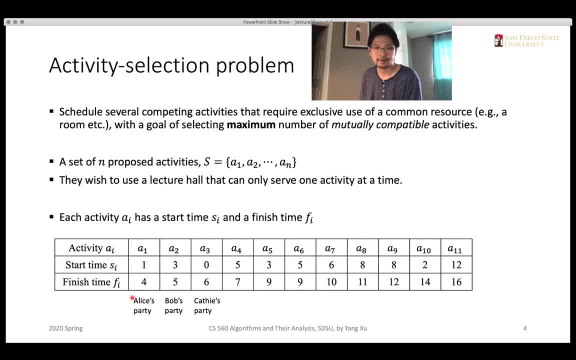 lecture hall. in this table we have the starting time and finishing time, 10 or while, and Flickr forcing to install everything within the time for each activities available. okay, and one more condition we provide is that we also sorts all the activities in increasing order of the finishing time. so if you look at the 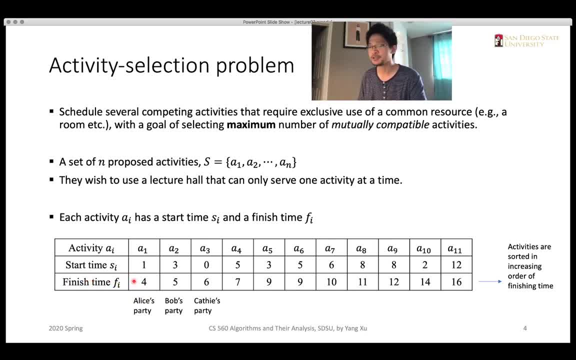 third row in the table, it's the finishing time for each activities. we it's already sorted: a1 ends at 4, a2 ends at 5 and a3 ends at 6 and a11 ends at 16, which you can think of it as 4pm, okay so. 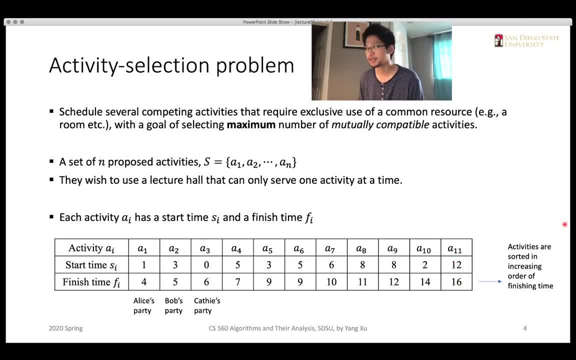 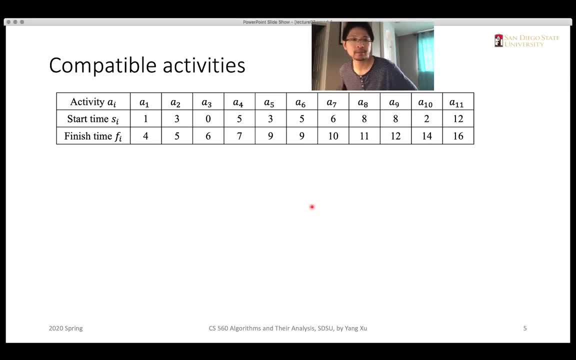 that's the setup of the activity selection problem. one important notation or concept is the so-called compatible activities, so we can use some notations to formalize this concept. so what are the? what are the compatible activities? how do we know that two activities are compatible with each other? okay, so if, given this, 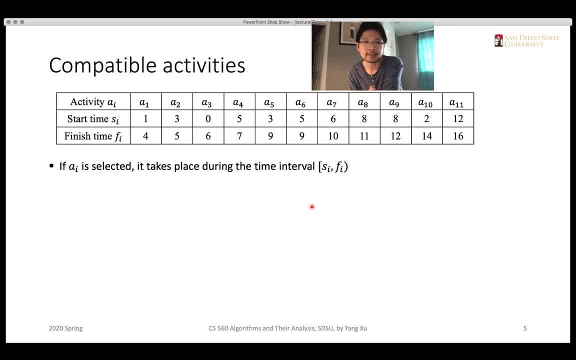 table. we know that when some activity, ai, is selected, it takes place during the time interval from si to fi. si indicates the start time, fi is the finish time. so we use square brackets on the left as an inclusive brackets and these round brackets on the right to add to indicates and: 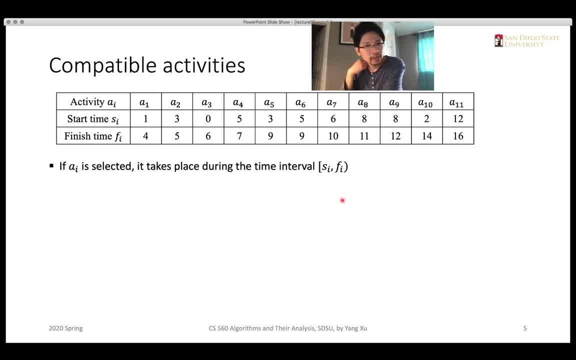 exclusive brackets. so we can use this mathematical notation to say that activity. i takes these segments on the time axis. okay, so we say that two activities, ai and aj, are compatible if their intervals say, this is the interval for ai from si to fi and the interval from aj from sj to fj. 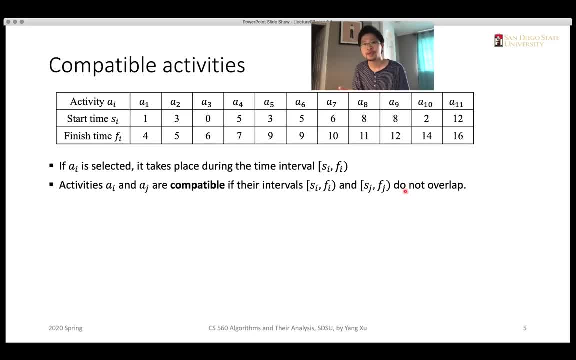 do not overlap. okay. so if after we put these two intervals onto the same axis, if these two segments do not overlap, then we say the two activities are compatible. this is quite straightforward notation that makes sense, right? so for example, in our case, in our example here, a1 starts from one and ends at four and a3. 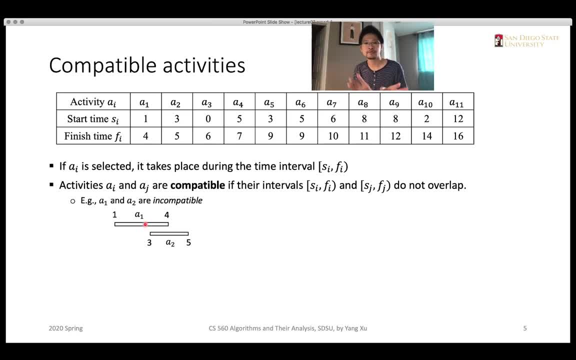 starts at three and ends at five. so if we put these two intervals onto the same axis, they certainly overlap from three to four, right? so that's why we say a1, a2 cannot. they are not compatible. therefore they cannot be scheduled at the same time. okay, so if we look at a1 and a4 and a4, according to the table, it starts at five. 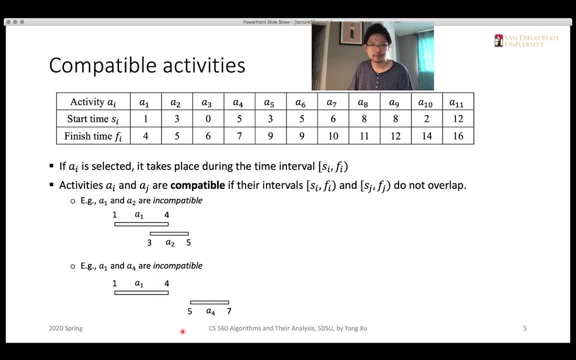 right, which is already after a1 finishes. so these two intervals they do not overlap. then we say they are compatible. okay. and more generally speaking, if two activities, ai and aj- are compatible, then we say either case should satisfy. so either si is greater than fj, so that means the starting time of activity ai is later than the finish time of activity aj. okay, 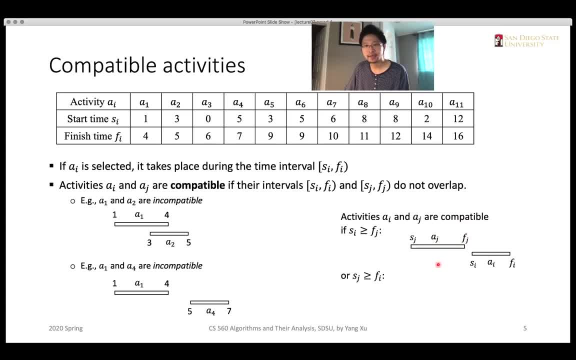 or the other case is satisfied, as i sj is greater than fi, which means the opposite way, the other way, the activity aj, it starts after the activity ai, i finishes. okay, so that's the two. uh, that's the more general definition of what uh a compatible activity, what two compatible activities are defined. okay, so now let's talk about the largest. 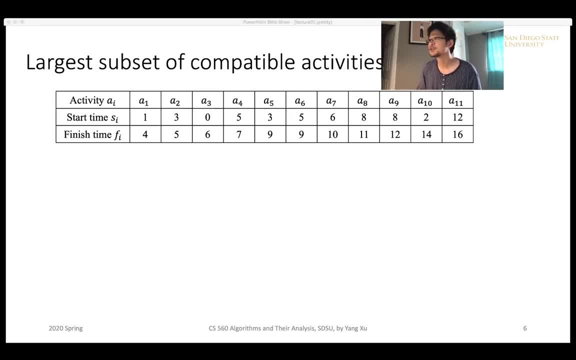 subset of compatible uh activities, which is the uh the goal of the activities selection problem. okay, so given one lecture hall right, we want to select as many uh activities as possible. so there are multiple. so if we don't place the constraints of maximum number of activities, we cannot. we can just arbitrarily choose multiple activities as long as they are compatible. 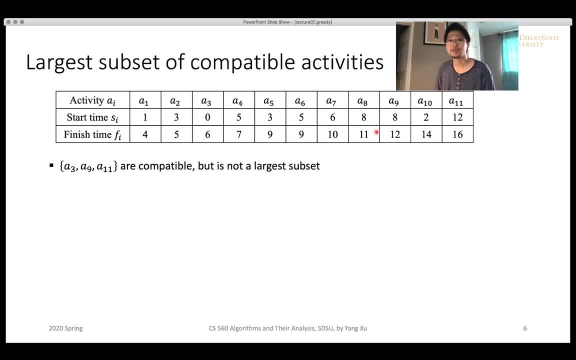 right. so for example, in the table here, a3 and a9, a11, they can be scheduled uh, at the same time. right, because uh a2, uh a3 doesn't overlap with a9 and a9 doesn't overlap with a11, okay, but even even though they are compatible, but they cannot be. 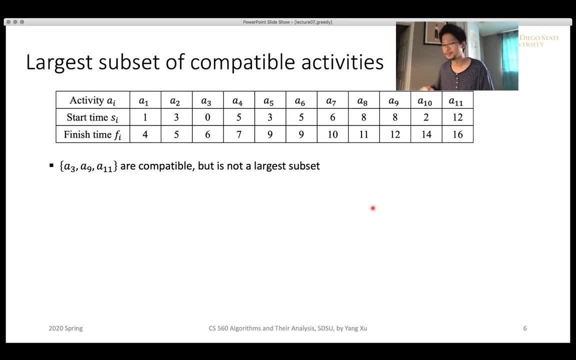 they are not the largest subsets. okay, because we know that we can select a1, a4, a8 and a11, and there are four activities scheduled, but they are also compatible with each other. and another example is a2, a4, a9, a11- okay, so these two cases make more use of their own. 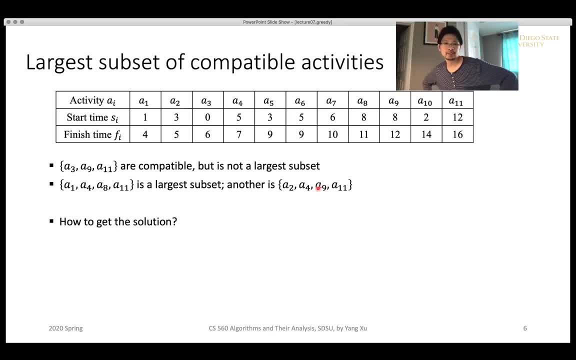 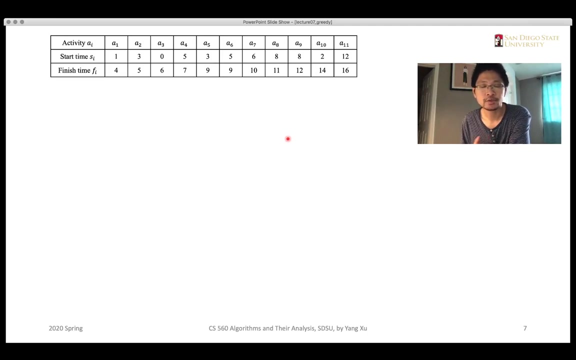 okay, so the solution- ultimately the solution is to the problem- is how to get the optimal solution. how do we get these solutions of four activities instead of the three activities or less? okay, so that is what we want to solve within this activity selection problem. now we can use this visualization technique to help us solve the problem of 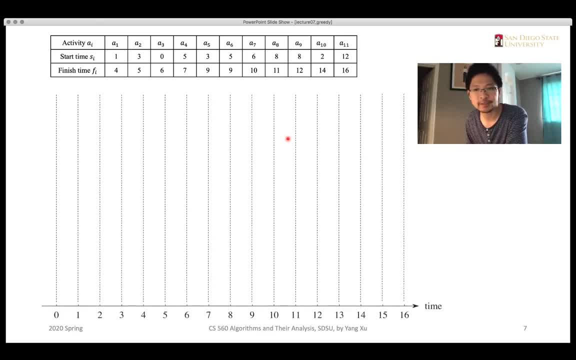 activity selection. so we can first draw this time axis and we lay out all the activities upon this figure by the increasing order of the finishing of the finish time for each uh activity. so we um put a1 first here because it ends at four. so we draw a little thin rectangle from a1 to a4 here and 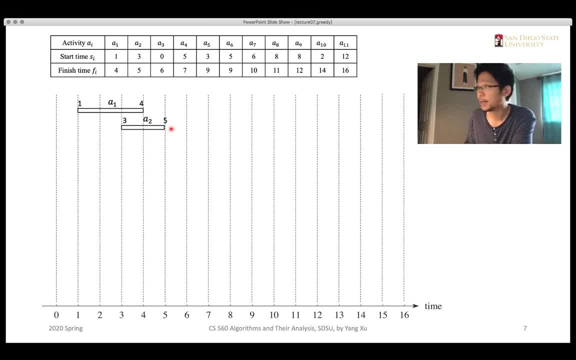 a2 ends at five, so that's where A2 lies, and next comes A3, which is from A0 to, which is from zero o'clock to six o'clock and so on. so we did this for all the activities. okay, so after we have all the activities now we can think about some questions like: 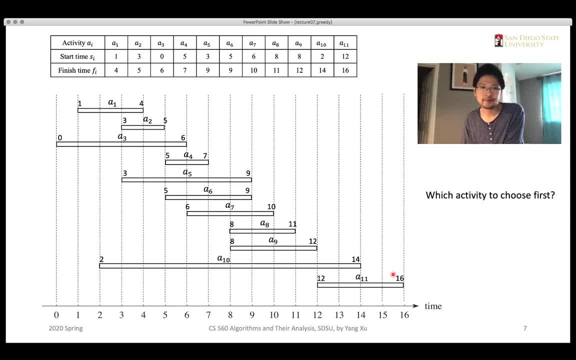 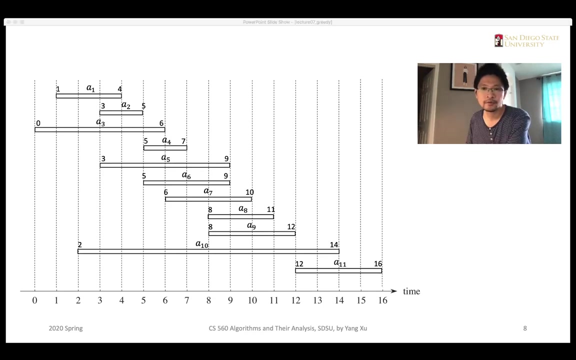 which activity to choose first and actually the activity that we choose first will determine what the next activities that we can choose or that are available to choose. okay, so, and choosing one activity will decide how much time that that is left for us to choose. for example, if we choose a1 as 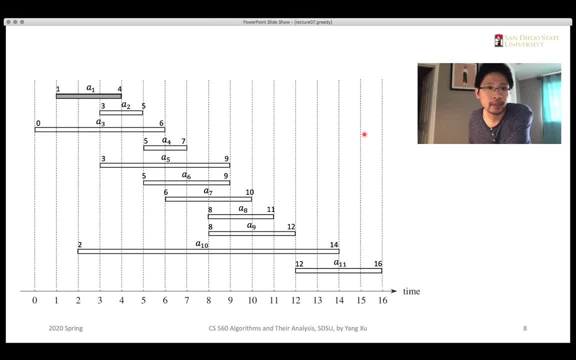 our first activity. then, after a1 is selected, then the, because the time period from 1 to 4 is already occupied. then we cannot select any activities that are incompatible with a1. okay, so in theory we can say that there are 16 minus 4 hours left that are available for other activities. right, because a1? 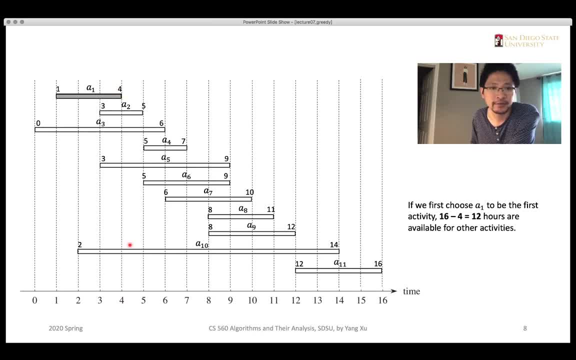 and at 4 we can only select activities within 4 o'clock to 16 o'clock after a1 is selected. right, so we can highlight the all the available resource, all the available time after a1 is selected in this column? and what if we select a2 as? 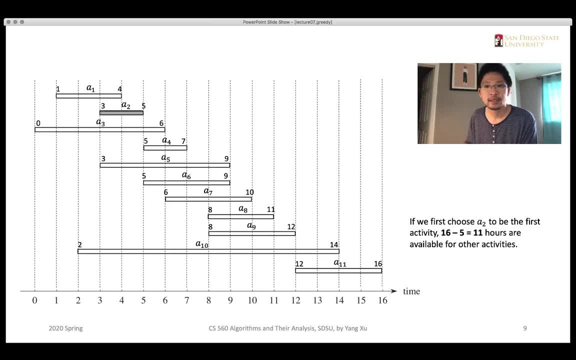 our first activity, then there are only 16 minus 5, which is 11 hours left, and that's the available time for so for select the rest of the activities, right? what if we select a3? then the time we have got left is from 6 o'clock to 16 o'clock. 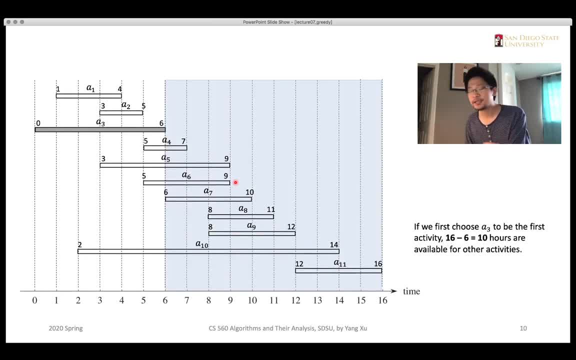 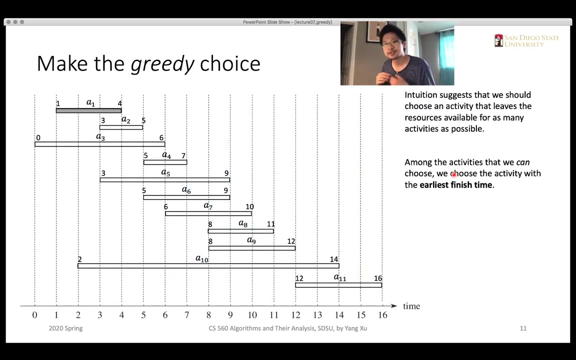 okay, so one of the ideas we her, So the idea now we can have from observing the consequences of selecting activities on the available time to the rest of the activities, is that we can select, we should select activity that leaves the resources available for as many activities as possible. right, because the from the 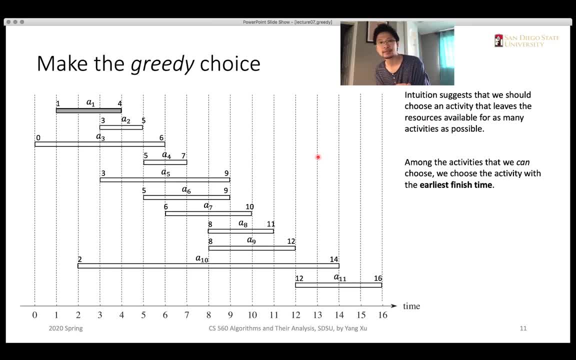 previous three examples, we see that after A1 is selected, there are 12 hours left, and after A2 is selected, we have 11 hours left, and after A3, we have 10 hours left. so in two tivis, picking which one is the best, right we it's. it's a. 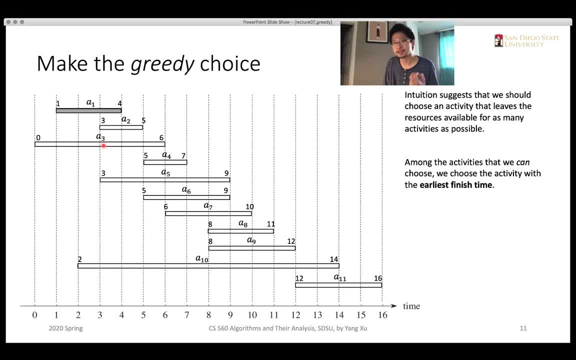 simple question. so we want the solution we want to suggest. we want the selection that leaves us as many hours as possible, because we want to select more activities. okay, so this gives us a greedy and a heuristic to choose ratios based upon an order from the previous example. so what would that mean? 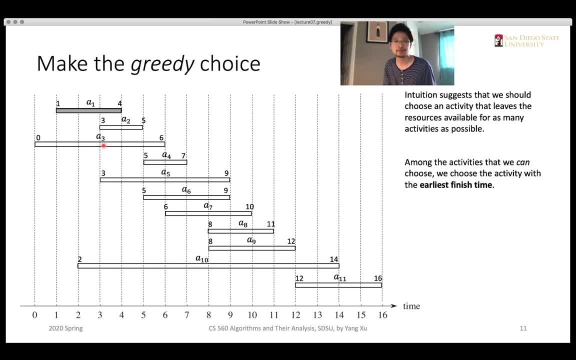 to make a greedy choice at each step to select an activity. okay, and this greedy choice is simply to choose the activity that has the earliest finish time, okay. so when we make the first choice, if you compare a 1, a 2 and a 3, a 1 has the 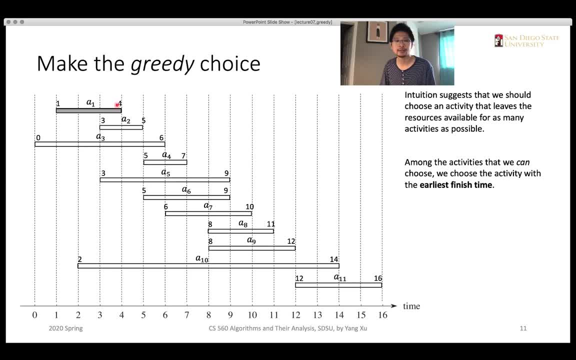 earliest finish time. it finishes at 4 o'clock, which is earlier than 5 and 6, and in fact a 1 is activity among all the activities that has the earliest finish time. so that's why we choose a 1 as our first activity. okay, after a 1 is: 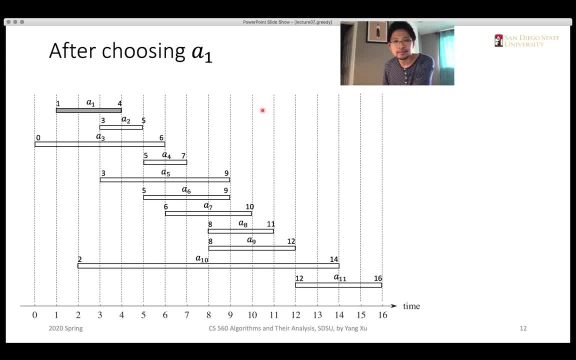 selected. now let's observe this figure, observe this time axis again. so, after a 1 selected, we have the rest of the hours, which is from 4 to 16, available. right, we should select the next activity amount of between 4 o'clock and 16 o'clock. okay. 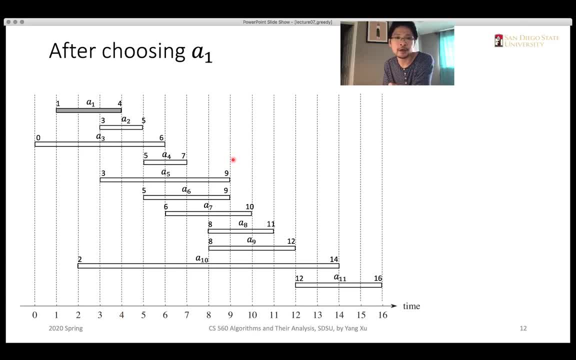 but not all the activities left are compatible with a 1. you see, I highlighted the incompatible activities with red color, because it is incompatible with a2. they have overlap, and a3 also overlap with a1, and so for a5 and a10, they all have overlap with a1. okay, so one of how do you see? 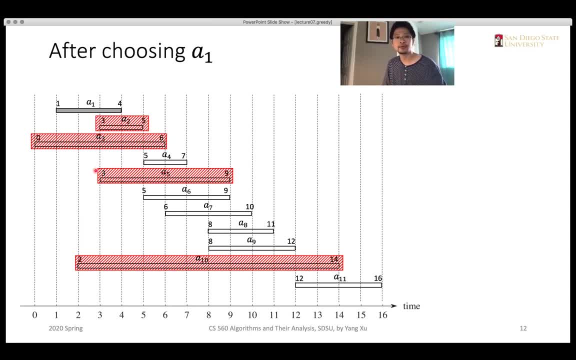 they are overlap. you just need to compare, you just need to look at to the starting time of a2, right, setting time is three o'clock, which is before the ending time, the finish time of a1, right. so as long as an activity, the start time of the activity, is earlier than a finish time of a1, then we can say that it's. 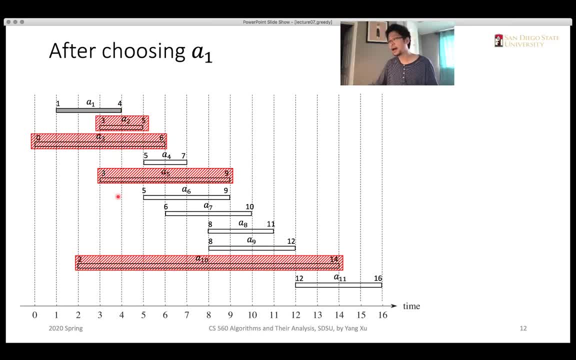 compatible with a1. so, anyway, the highlighted activities are crossed out, they're removed from our list. we cannot choose from them because we already choose a1. okay, so, among the compatible activities, what's left? the non-highlighted ones? what is our selection? well, we need to stick to the our heuristic, our, our greedy heuristic. 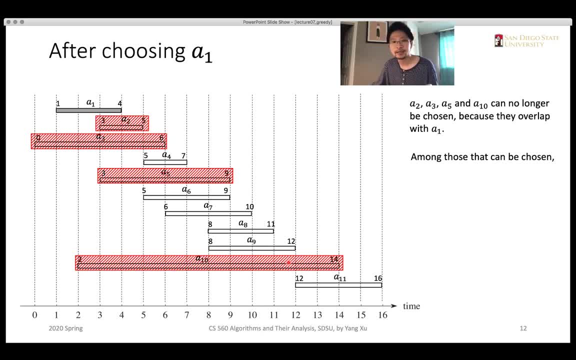 right. we want to choose the activity that has the earliest finish time among all the compatible activities, and we found that we can find that a4 has the earliest finish time. it finish it at 7 o'clock, which is earlier than 6 a 7, a 9 and a 9, a 8, a 9 and 11. so that's why we 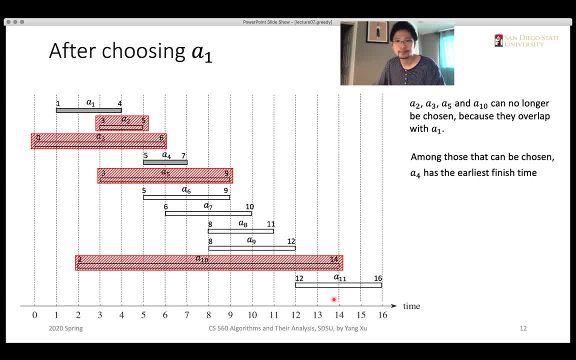 need to choose a 4 in now in this case. okay. so after choosing a4, we need to do the same thing. we need to first look at which activities are不會成功 available for being chosen for the next one. okay, we find that's a 6 and a 7. they. 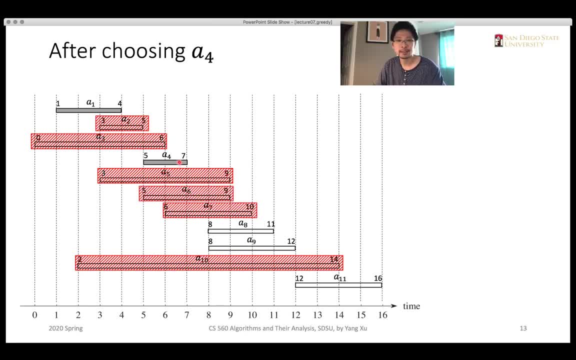 are incompatible with a 4 because they overlap with a 4, so we cannot choose them. therefore, we must choose from a 9, a 8, a 9 and a 11, and the policy is that we need to select the one with the earliest to finish time, which is a. 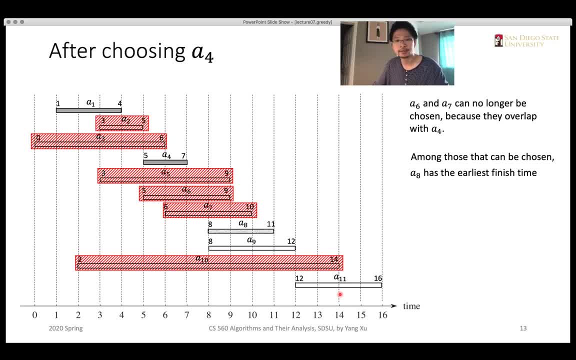 8, and then we choose a 8 and a question. the next question means the same. we want to avoid choosing the incompatible ones, right? so a 9 is crossed out and we need to choose the compatible choose among the compatible activities and in the last case, we only have a 11 to choose from. so we need to choose a 11 and 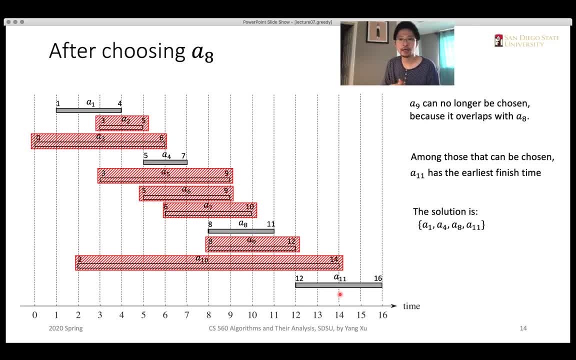 that's it. we have a solution which is a 1 to a 4 to a 8 and a 11. that's our final solution that gives us a complete list of activities based on our strategy of choosing the activity that has the earliest finishing time. okay, so that strategy is a greedy strategy. okay, because we just want to. 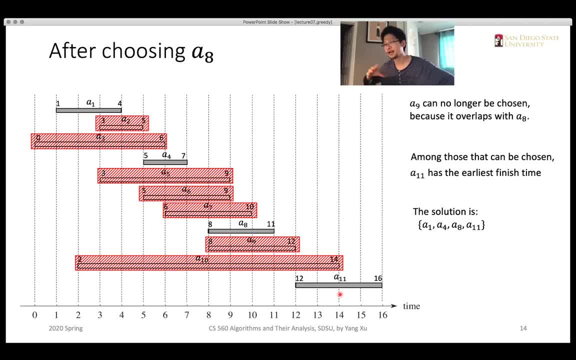 solve. we just want to have a activity that gives us the locally best solution, but we don't know whether this is true globally. well, it turns out that in the case of activity solution- activity selection problem- this greedy strategy will give us the best solution. okay, but it is not the only way to solve the 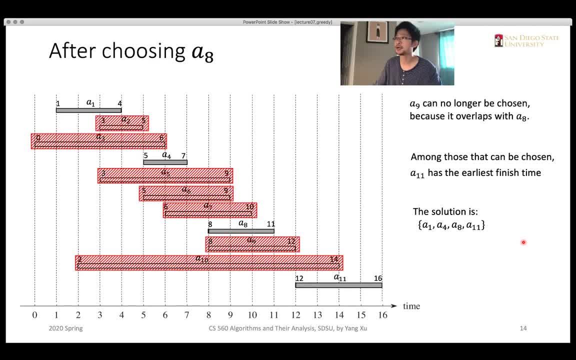 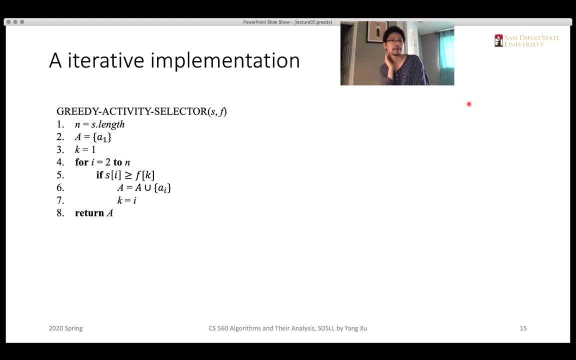 problem. we cannot of other heuristics in later slides, and first we can look at how we implement these greedy strategies using pseudocode. okay, so here is a, an iterative implementation of the algorithm. okay, so looking at the pseudocode, this procedure is called greedy activity selector. okay, and it. 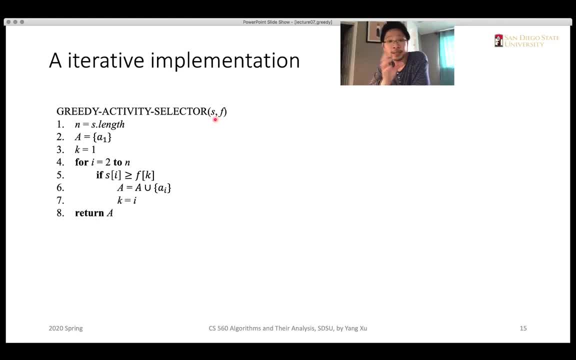 takes inputs, the S and F areas, so as as remember, it records the starting time for all the activities and F records all the finished times, uh, for all the activities. and then we assume that we have n activities to select from. okay, so we also assume that input activities. they are already sorted in increasing order of the. 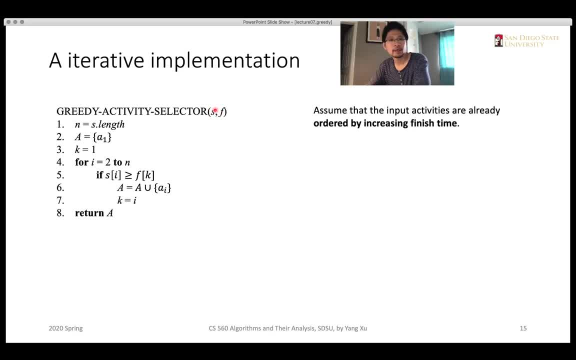 finish time. okay, so that's our assumption, and in line one we just record the number of activities, okay, and we store a1 into a, a set, okay, into a set called capital a, and this is the set that will finally return. so this is the results that we uh, this is the variable that we will store. 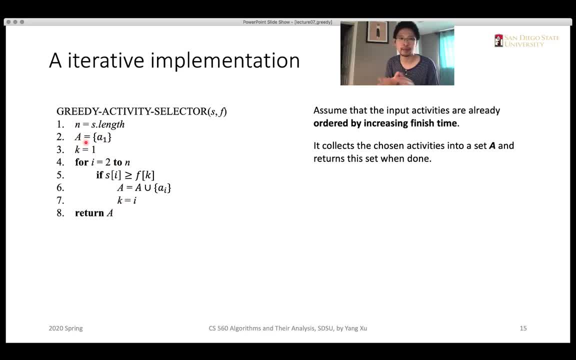 order, our all of our final schedules, our results okay, and a1 is automatically selected because a1 has the earliest. because we already saw, we assume that all the activity are sorted in increasing order or finish time and then we will define some variable k. it starts from one and this k is the index. 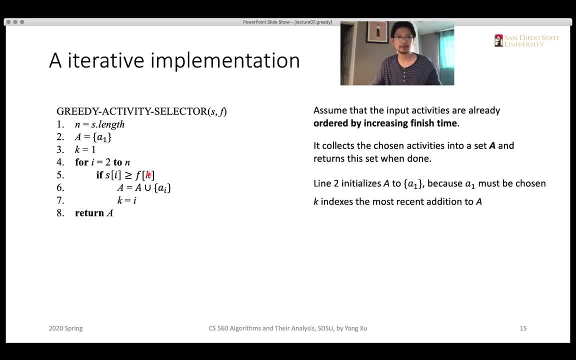 for the most recent addition to a, or in other language we can say: in other words, we can say: k is the index for the most recent selected activity, because we just selected activity one to a, to the capital a. that's why we let k be one. so k indicates that a1. uh, k equals one, indicates that a1 is the first activity. 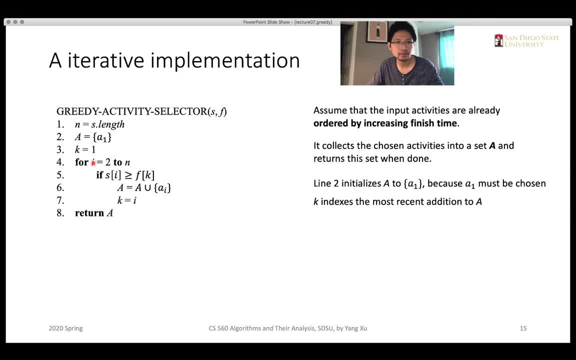 we select. okay, then we will go through. use a for loop to go through from to go through activity 2 to activity end. we will go through all the activities to a, then after the first one, just for a minimum, then using all the activities wecaves for nothing else. okay, then, to then go after wecaves for all the activities we. 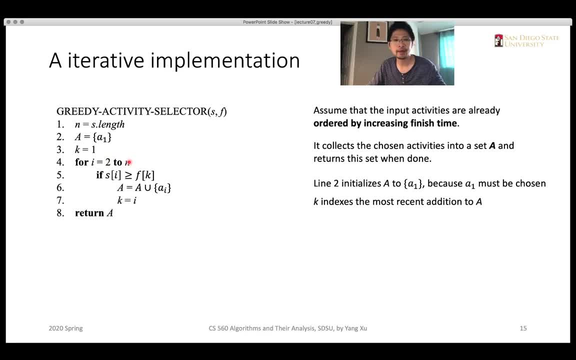 go through all the activities and within the body on the for loop, we use a if condition to check to find the compatible activities that finish earliest. okay, so we will compare the starting time of activity i with the finish time of activity k. so k is the most recent activity. that has been. 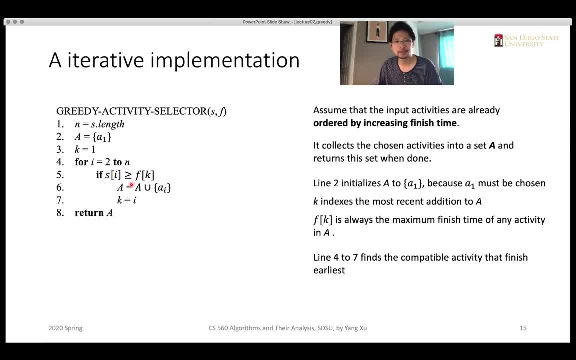 added that has been selected. so, among the rest of the activities, we want to compare the starting time with the finish time of k. so if the starting time is later than the finish time of k, then we will add the activity i into the into the final solution a okay, and then we will jump towards jump to the next uh. 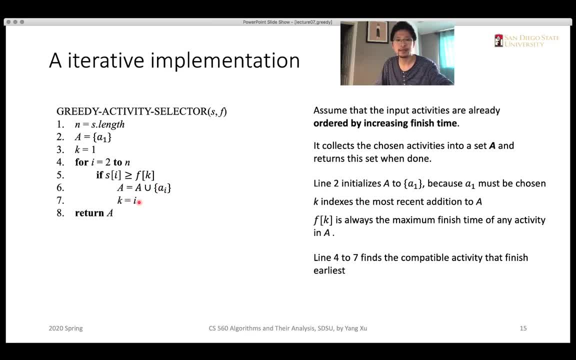 activity. we will let k, let let k be i, which is the newly selected activity. okay, and finally, a is returned okay, so in this code, k is the index of the most recent selected activity and it is always the maximum finish time for any activity selected in a. okay, and that's based on the fact that 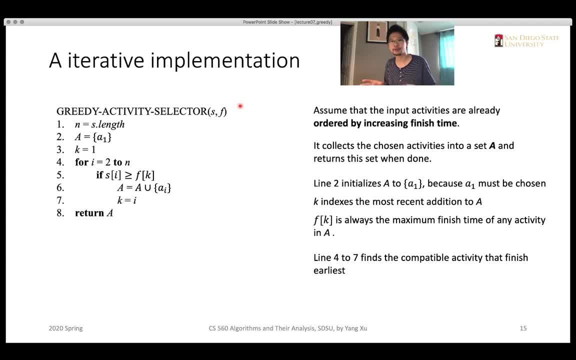 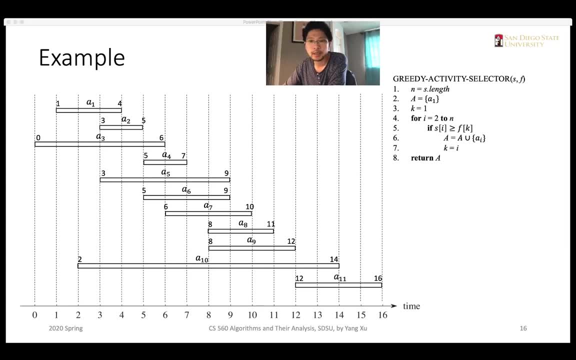 all the activities in s and f. they are already sorted in an increasing order of finishing time. now let's run this greedy activity selector procedure using our input example. so all the activities the s and f table are like this are indeed are demonstrated by this figure. okay and uh. 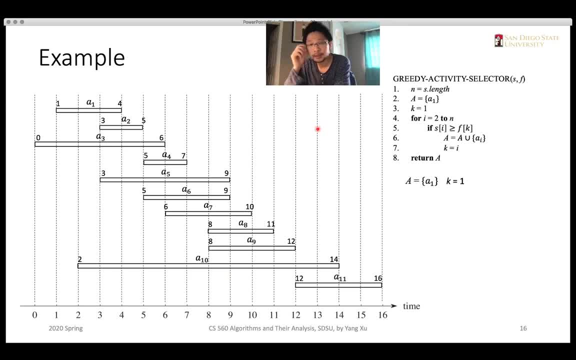 we, according to the procedure, a- the capital, a- all the activities. it is initialized with activity one, it is automatically selected and k starts from one. okay, and let's go into the for loop. so i will start from two, okay, and if we look at a two, the starting time is: 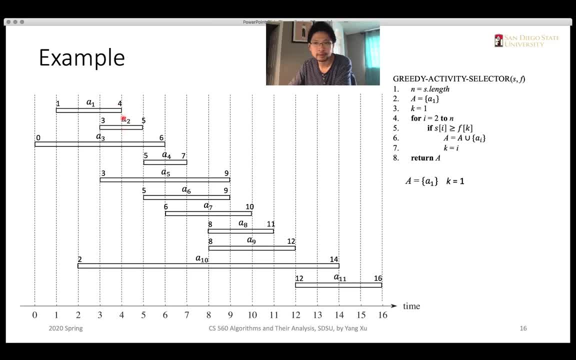 earlier than the finish time of uh, a1. right, so it is earlier. it is not satisfied. uh, the if condition at line five is not satisfied. for i equals two, so we will skip i equals two and for i equals three. as three is zero, it's also smaller than um than the finish time of a1. okay, so a equals three is. 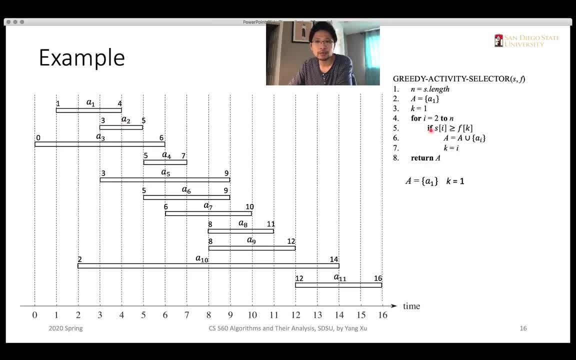 also skipped. and when i equals four, it is the first time that the starting time is smaller than a than the finishing time of a1, so a4 is selected, okay. a4 satisfy uh. s4 is greater than the finish time of of a1, so a4 is selected okay. 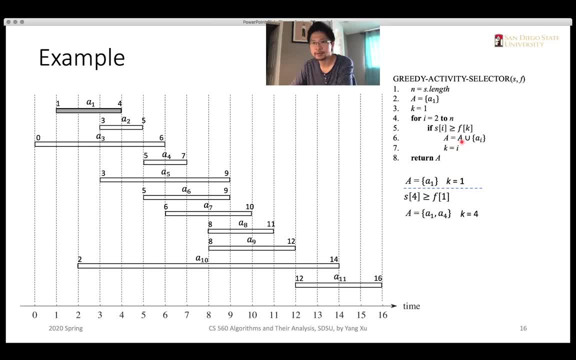 so a becomes the union of a old a, the old previous a and the new a4. so a is the set of a1 and a4, and k is being assigned a new value of the newly selected activity. k equals four after a4 is selected. so from the next iteration of the for loop i will start from five. 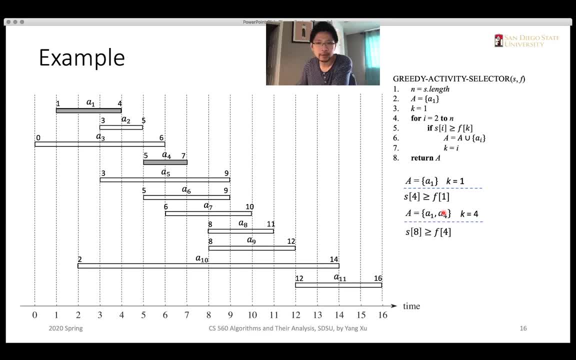 okay. so when when i is five, it is incompatible with a4 and i6 is also incompatible and for i7, also incompatible when i equals eight, it satisfies that its starting time of i8 is smaller, is greater than, uh, the finish time of a4. so 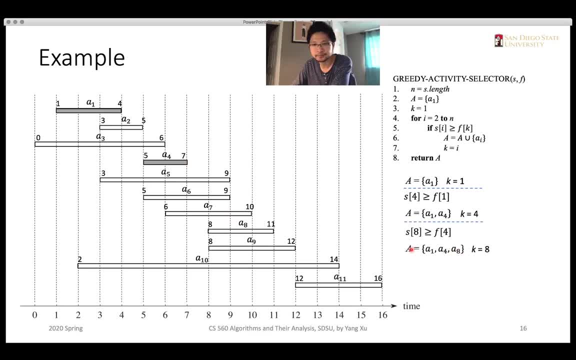 a will be added to the activity, a to the set eight and i will. k will be assigned uh, eight, and after eight, a8 is selected, we go through. i will go to a9 and a10. they are all incompatible and when i is 11, it's compatible, so that therefore, a1 will be selected. 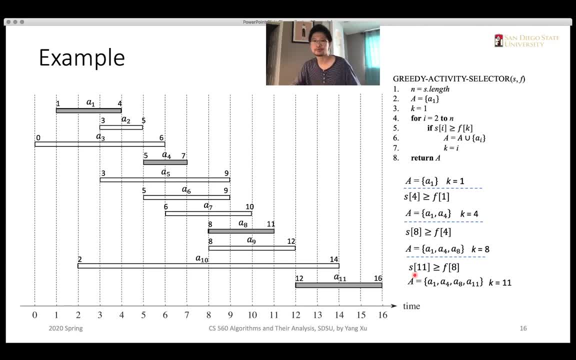 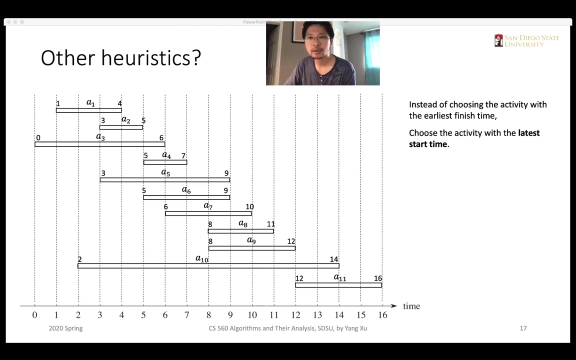 and that's the process of how this procedure runs on our input example, and it's quite straightforward, it's a very this procedure describes the way we think about this problem: using the greedy search, using the greedy strategy to select the next available activity. so here i would like to mention that we can use- actually use- a different heuristic. 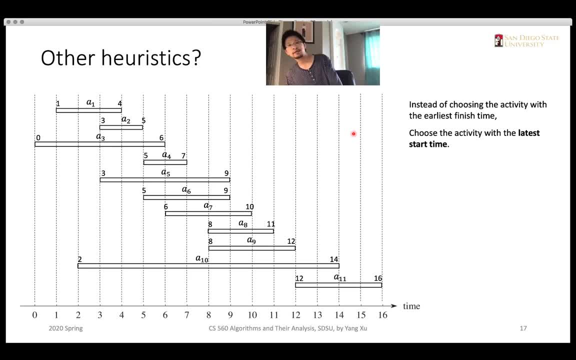 to implement a greedy algorithm. so previously we have choose the. we choose the strategy of selecting the activity that has the earliest of finishing time, because the idea is that if an activity finishes early, then we will have more time available for the rest of the activities. so we can think of this problem differently, like 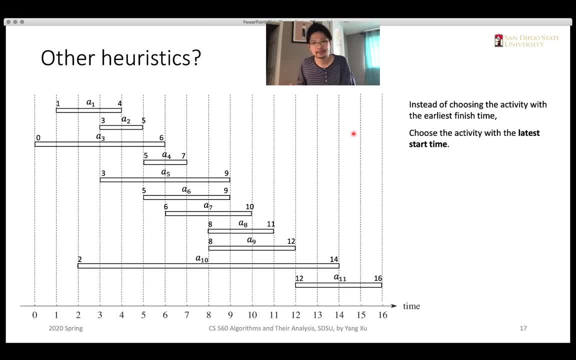 what if we choose the activity that has the latest start time right? if it starts late, then that means we we should have more time before that activity starts right. so that's just the opposite opposite way of thinking. but it also has the same idea of um preserving more resources for the 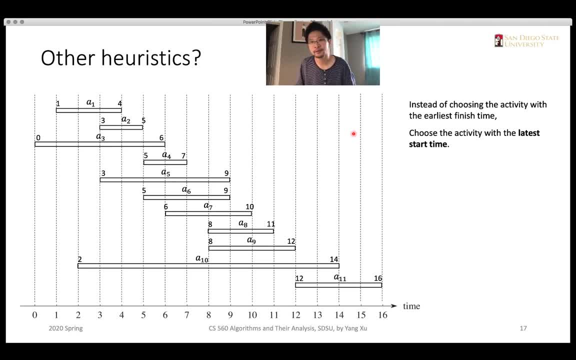 for the activity, for the uh activity that are left right. so what if we choose to implement the algorithm using this uh different bar, similar uh strategy? we cannot kind of also solve the problem right? so what if we choose activity among this same data, among these same um? 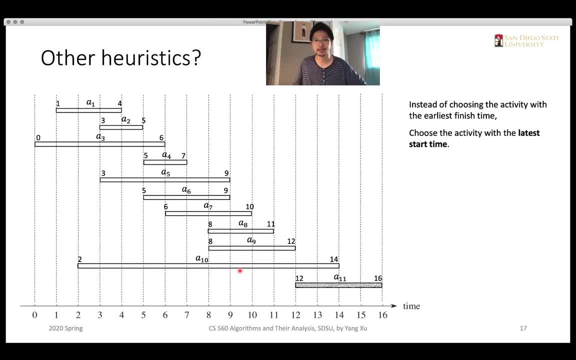 inputs. what if we choose the activity that has the latest starting time, let's say start with, for example? we choose, for example, let's say a11, always at the start time. the statt first, which is the first wave after a11, will be slower 고 going forward. 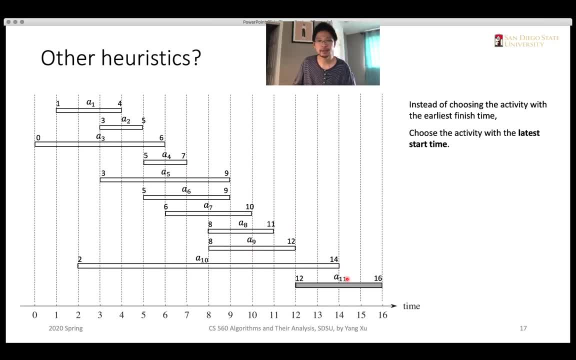 then out to a fashion. one at a11 will be: choose at first, right. then we go backwards instead of going to forwards. we will go back to see the all the activities that are left, which one we can choose. we can select from a4, because it is compatible with a9 and also has the latest start. 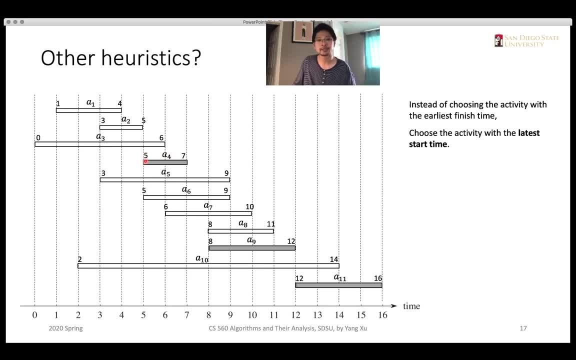 time, and after a4 is selected, we can select a2 and it. it seems correct in this situation. right, but we are missing something, because this input data, they are sorted by the order of um finishing time. right, what if we so, if we want to use the start time as our heuristic. 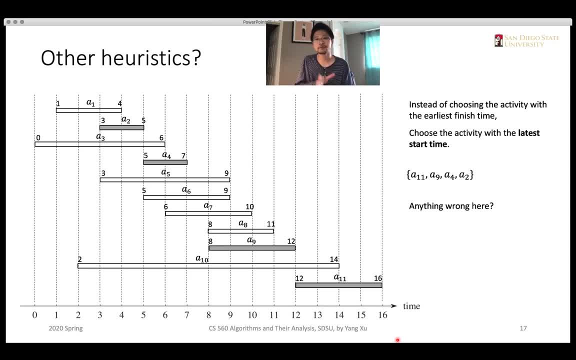 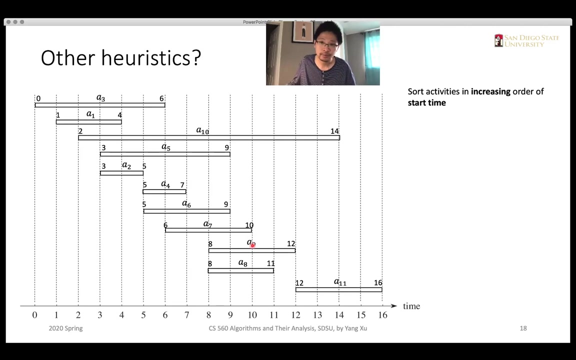 we need to sort events by the increasing order of the start time instead of finishing time, and we are lucky to get this optimal solution from this data. but if the, if the events, if the data, they vary a bit, we might have a wrong solution. okay, so the actual way needs to uh, the the the correct way needs to be like we first in. 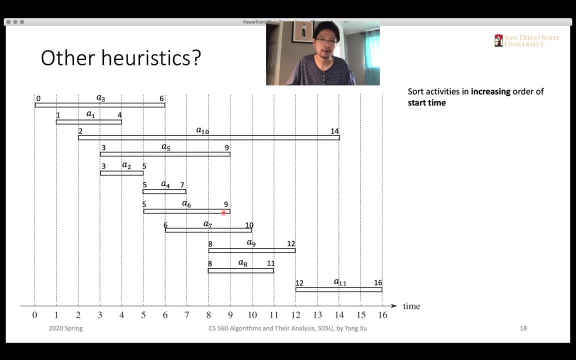 sort all the activities in increasing order of start time, and then we choose the, the, we choose the last activity, right, and then we choose the activity with the latest start time among the compatible activities, which will give us, uh, basically a bit different solution, but in this way it is guaranteed to be correct, okay, so, um, that said, the idea is that the input 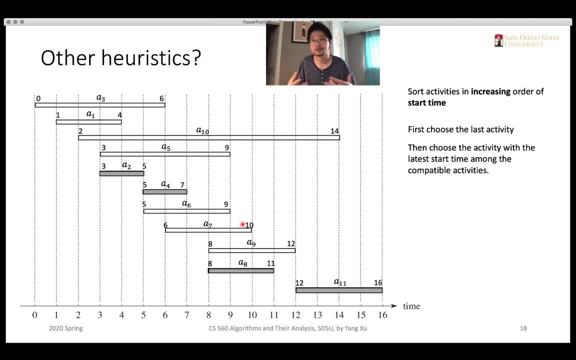 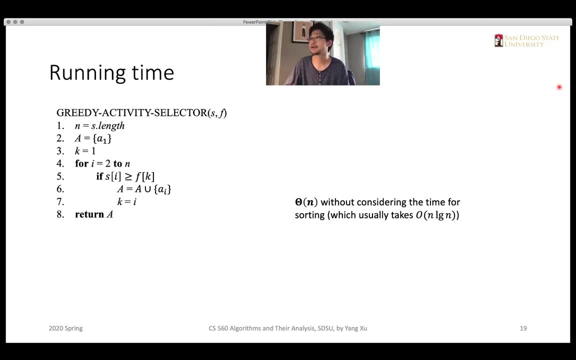 how your input is organized should be connected, should be related to the strategy you choose to use uh, to the heuristics you choose you use for the greedy uh strategy. okay, and lastly, let's analyze the running time for the um uh for the greedy activity: selector activity uh, selector uh procedure. so it's quite simple. 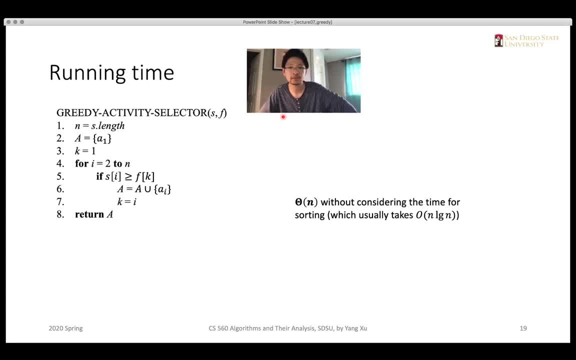 there's just one for loop in this algorithm, and that's why you can directly think of it as a linear running time bounded by big theta of n. okay, but this is without considering the time for sorting the all the inputs, s and f right all the activities. they are sorted by the increasing. 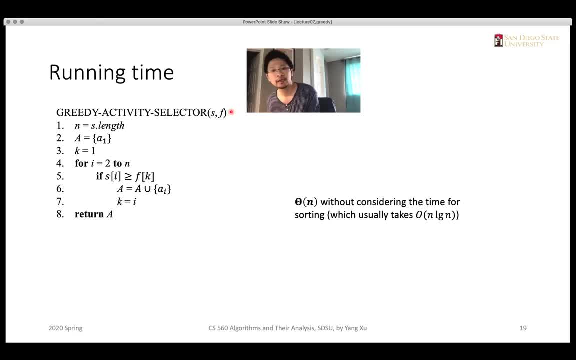 order or finishing time. so if we use a, an efficient sorting algorithm, to sort all the inputs data, all the input areas, then in theory it should take us n times logarithm of n. so that's something you should consider if you want to analyze the running time in a comprehensive way. okay, 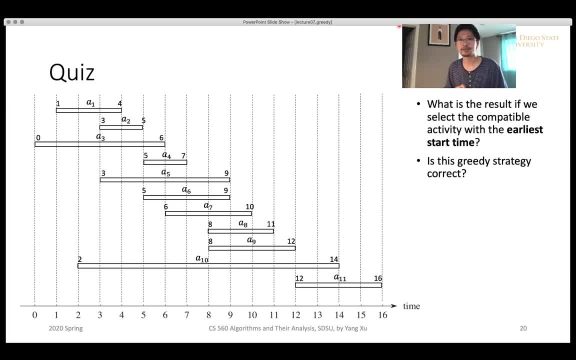 okay. so now let's have a quick quiz. uh, about the greedy search, the greedy algorithms for activity selection problem. so the question is: given this inputs, okay, given all the activities, information here in this plot, so what is the results? what will be the activities that you select if the strategy is to 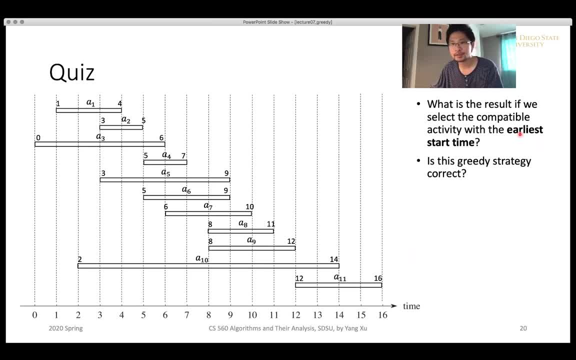 select the compatible activity with the activity that you select, okay. so if you select the compatible activity with the earliest start time, okay. so this is a different strategy from what we have been talking about so previously. the example in the slide is there's is the strategy to select the. 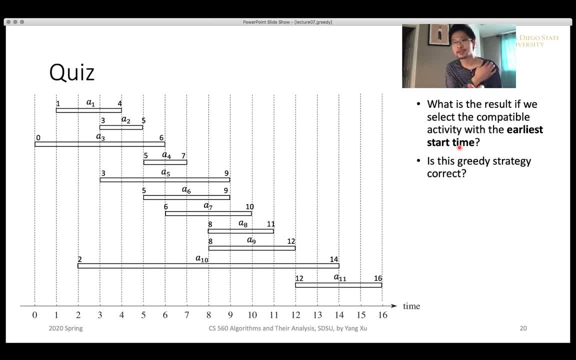 earliest finish time. right, but this time, what if we select activity with the early start time? uh, please take out a paper and write down the results of uh selecting the earliest start time, and uh also put an answer about whether this gradient strategy is correct or not. okay, and uh, i will open up a submission window on blackboard today and uh and you should submit it. 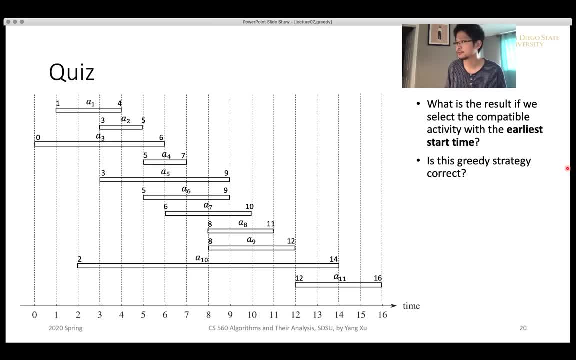 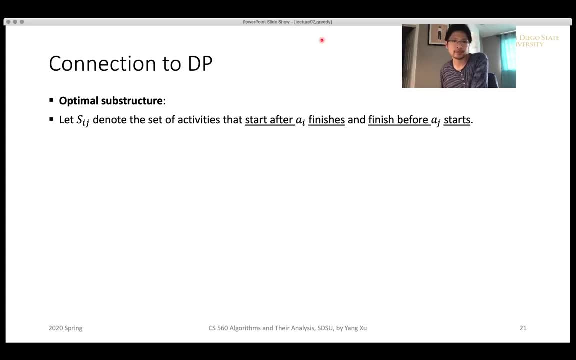 by the end of today. okay, so that's a really quick quiz problem. now let's quickly, uh, talk about the connection between greedy algorithm and dynamic programming approaches. so one of the characteristics of dynamic programming algorithm is that the problem should demonstrate some optimal substructure, so, which means the solution to the optimal solution, the the solution of the optimal. 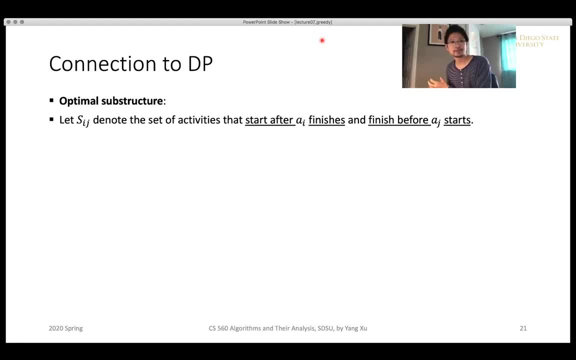 solution of the original problem consists of the solutions of sub problems. okay, so that's also. this property of optimal substructure is also demonstrated in this activity selection problem. so if we let this notation big s with subscripts s and j to denote the set of activities that starts, 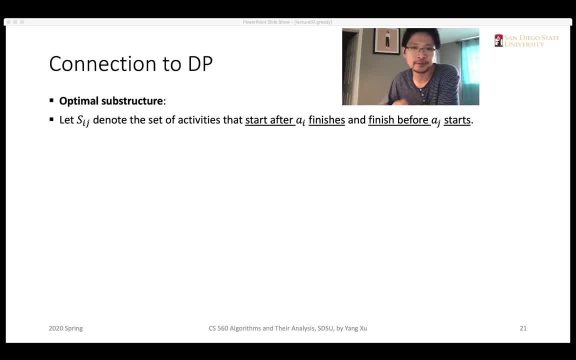 after activity ai finishes. so this i indicates we are considering all activities after activity ai begins after a i finishes, and this subscript j indicates we are considering all activities before a j starts. so we are considering a interval between active i and activity j. so let's s i j to denote. 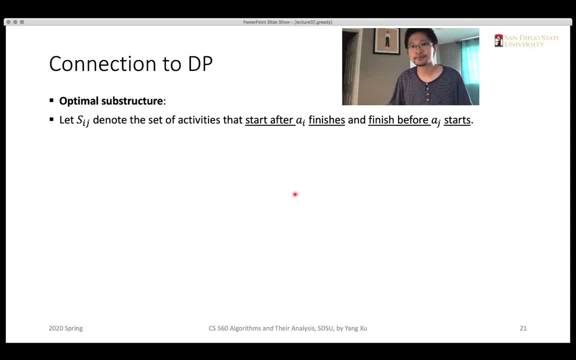 all the activities between a i and a j. okay, and we wish to find the maximum subsets of mutually activities within s i- j and we let the capital a with subscript i j to indicate such a maximum subset of mutually compatible activities in s i j. okay, so the problem is to um solve this. 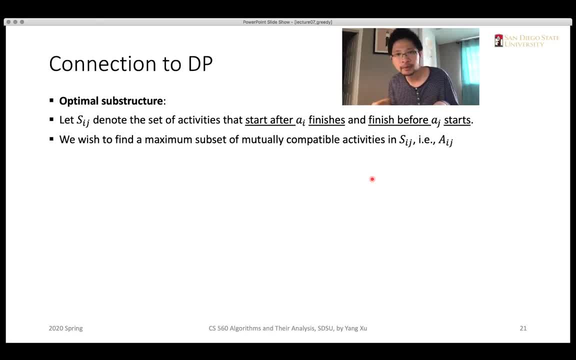 to to find the maximum number of common uh mutually compatible activities within s i j. okay, so let's say, if um a k, one particular, one specific activity, a k is in the uh mutually compatible activities, that is to say, a capital, a i j. so if a k is in the 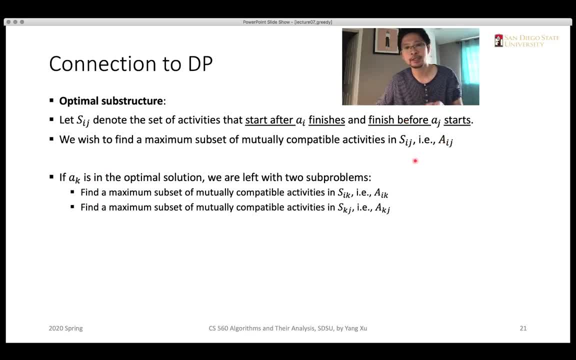 optimal solution, which is capital, a subscript i, j. then we are left with two sub problems. okay, we want to first find a maximum subset within s i k. right, because k is between i and j and the k splits the s i j into two parts, which is s i k and s k j. so we want to solve the problem within s i k. 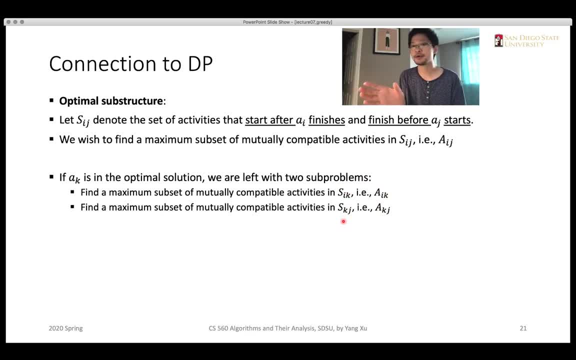 and get the solution with a i k, and we also want to solve the problem of s k j and get the solution of a k j. okay, then the final solution is to find the maximum subset within s i k and get the solution. okay, then the final solutions of a i j is the union of three parts: first, a i k, second, the- the specific 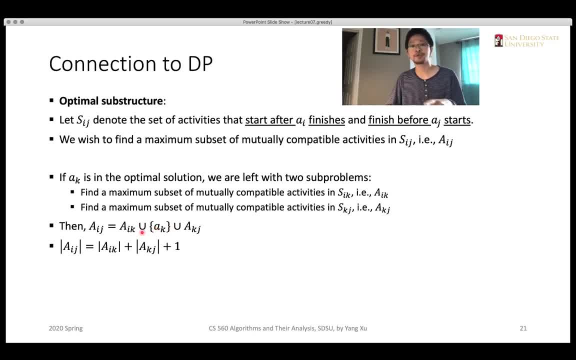 the specific event, a k uh, which itself consists of which itself um as a as a set, and the third part is a k j. okay, and the number and the size of the set is the size of a i k plus the size of a k j plus one. so this is a very typical, optimal substructure, okay. 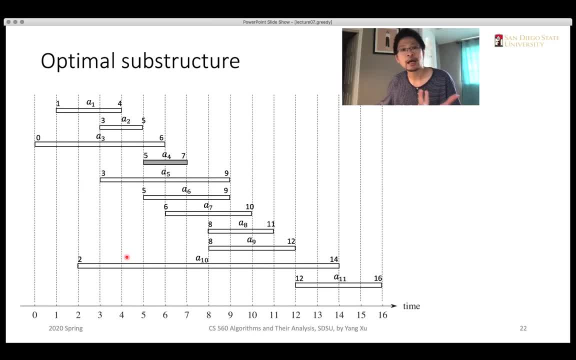 so if we consider this optimal abstracture, visualize it within this inputs, uh, figures here. so if the the considering a problem, the problem is to find the maximum subsets of compatible activities within the range of 0 and 16.. okay, so our problem can be written by: 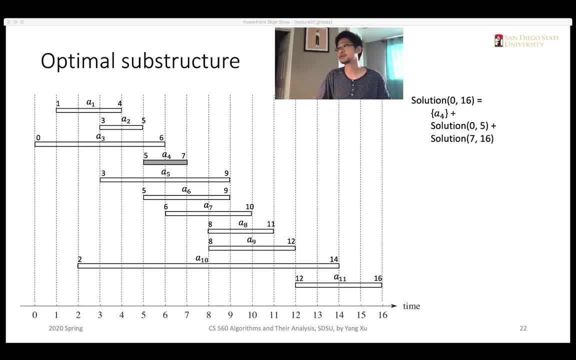 this solution of 0 and 16.. okay, so this 0, you can think of it as the i, the 0 can, you can think of it as the i and 16 is our j. so the problem is to solve the, solve the ring, the the original problem is with between the range of 16, 0 and 16.. so what if 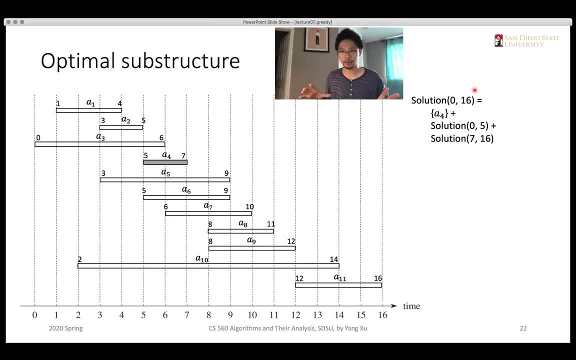 if a4 is in our solution, so that's if if a4 is within our final solution, then A4 actually divides all the activities into two parts. right on the right part are all the activities that starts after a4 finishes, and on the right are all the activities that start after a4 finishes and on the 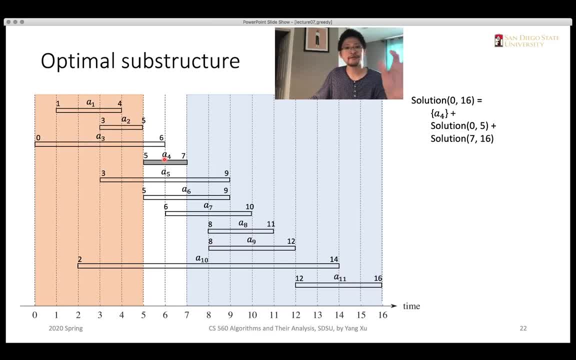 activities, that's starts before that finishes before a4 starts. so we want to solve the two parts right. individually, we need to get the solution from the range between 0 and 5 and the solution between the range and 7 and 16, and then we need to combine the two, the three parts, as a solution to our original. 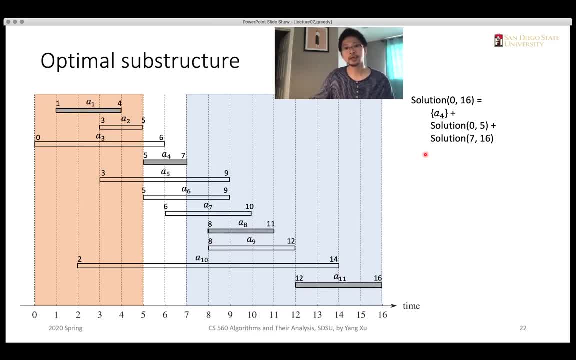 problem, okay. so in this case, if we solve between 0 and 5, we will have a 1. if we solve between 7 and 16, we will have a 8 and 8, 11, okay, and the final solution will be a 1, the union between a 4, a 1 and 8, 8 and a 11, which is 1, 4, 8, 11, okay. 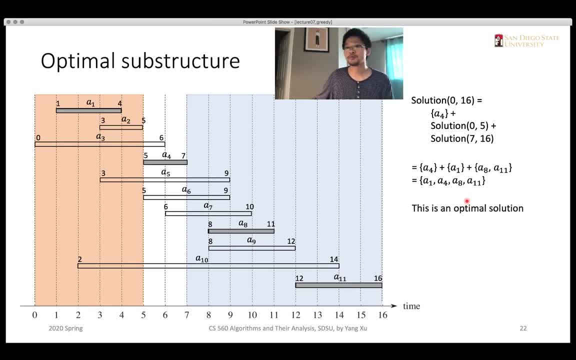 and that's just one case. so what if you and this turns out to be the optimal solution? okay, and what if we choose a 5 to be the activity in the middle? then a 5 would divide all activity into two parts. similarly right, and we need to solve the two ranges individually. from a 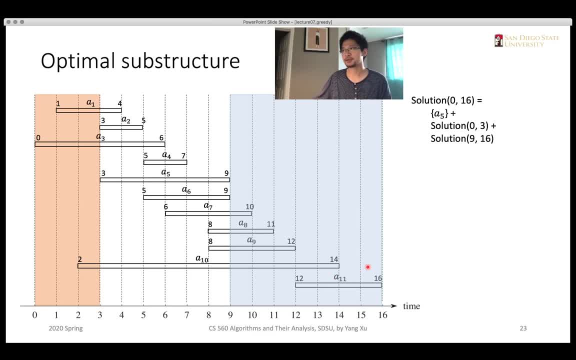 0, from 0 to 3 and from 9 to 16. okay, solving 0 to 3 will give us nothing, because there's no compatible events, and solving between 9 and 16 will give us a 11, so the results will become a 5 and a. 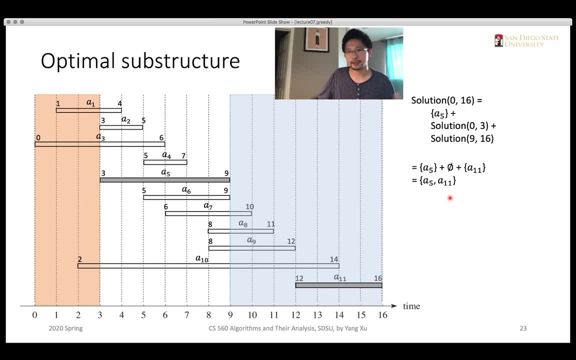 11, which is obviously not a optimal solution. okay, so, having shown these two examples here, what I want to say is that this is a because the problem demonstrates optimal substructure. if we want to obtain the optimal solution, we need to go through all possible ways of. 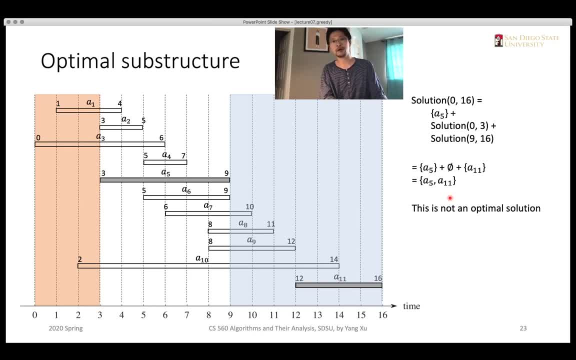 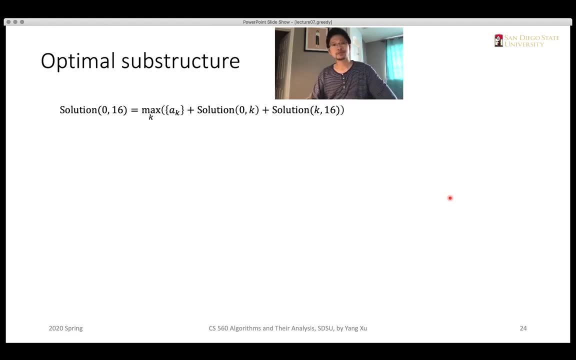 this optimal substructure, we need to solve all possible sub problems and this is a very typical dynamic programming approach, dynamic programming way of thinking. so to summarize a bit The solution, the original solution of between 0 and 16 is the result of choosing the k and solve the left part between 0 and k and solve the right part between k and 16.. 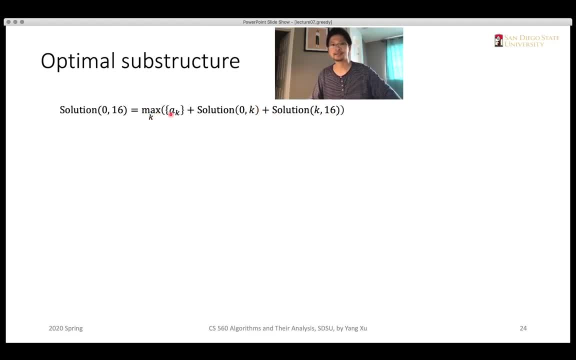 And we need to choose the k that maximize the combination Right. Not all k's gives us the optimal solution We want to solve. we want to iterate over all possible k's and solve the final and get the k that gives us the optimal solution. 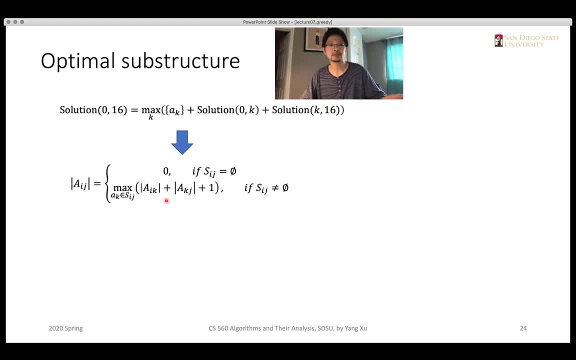 So this is a very typical dynamic programming way of thinking. So if you connect this to the original, to the previous lecture, to our either matrix chain sub-problem, matrix chain multiplication problem or the rock cutting problem, Okay. So If we write this into a different notation, so if we abstract the solution notations with the a of ij, 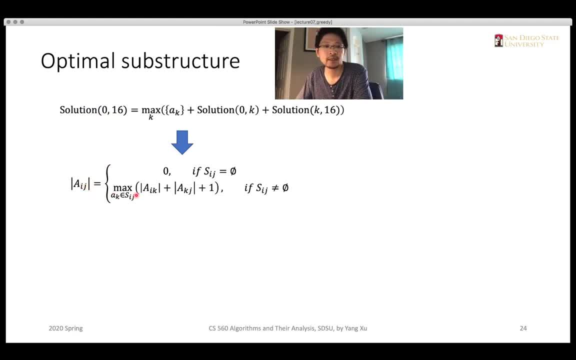 then the a of ij is the maximum among these combinations in which a k is a one activity among the subset of s ij. Okay, And we can further use the 2D array notation To further simplify this optimal substructure, right. 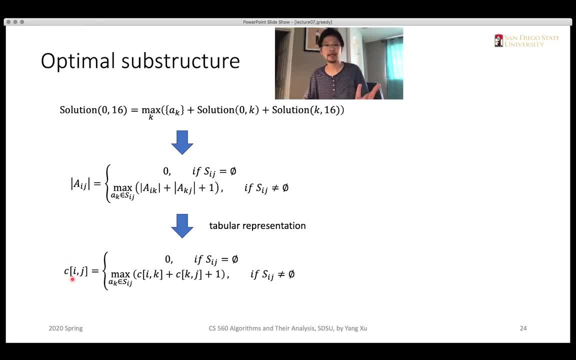 We can use c ij, which is an element of a 2D array, to indicate this a ij, right, So it finally becomes a dynamic programming approach. Okay, But I would like to point out that this is an overkill. So in a case of activity selection, 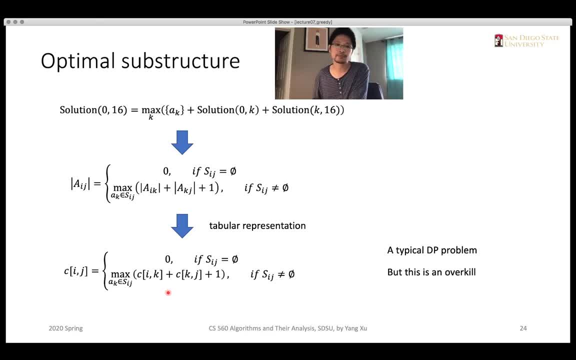 Problem. we don't need to solve all the sub-problems in order to get the global optimal solution. Okay, We just need to solve. We just need to use the greedy approach or the greedy strategy to choose the locally best one. Okay, 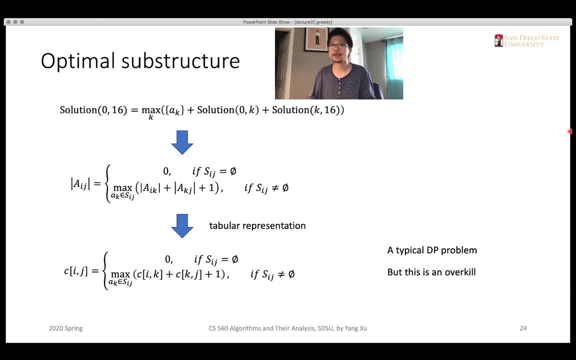 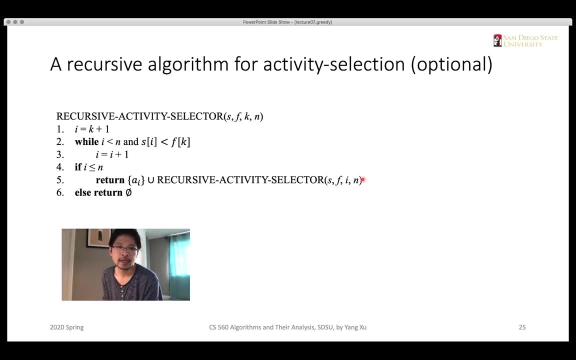 And we will go back to the connection between dynamic programming and greedy algorithms later, When we Finish up this lecture. Okay, So, lastly, let's look at a different way to implement the activity selection, The greedy algorithms for solving the activity selection problem. 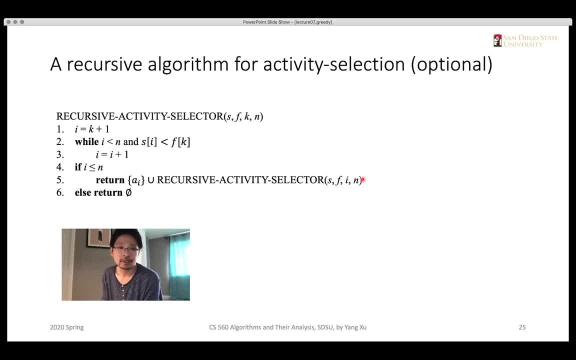 So this is a recursive way, recursive algorithm of solving a problem, Which is different from the iterative way of solving it. but we'll see how running this algorithm will result in almost the same results and how the recursive calls selects the next available activity. that is that satisfy the greedy strategy is very 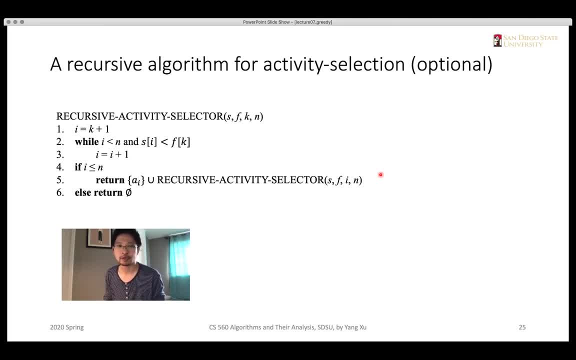 similar to the how a, an iterative algorithm, does. okay, so this is how the recursive algorithm looks like. it takes, in addition to the S and F parameters, which contains the starting time and the finishing time information, it also takes two integer numbers, K and N, to indicate the range of the problem. that 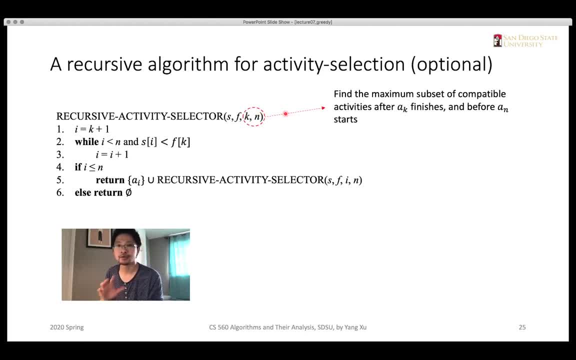 this algorithm will solve. okay, so the K indicates that the procedure will find the maximum subsets of compatible activities after the activity A finishes and before the activity an starts. okay, so it will initialize the a integer i as the next symbol activity right after activity K. okay, and it uses a while loop to increment I. okay. 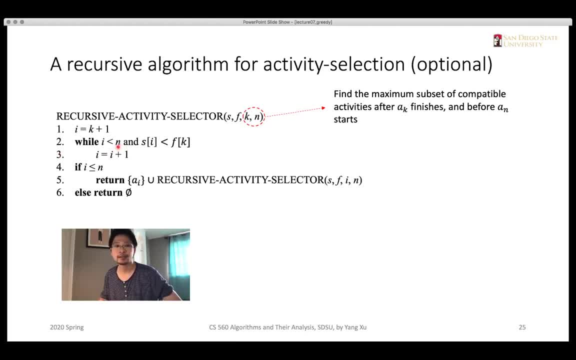 and the while loop will break if either one of these two conditions breaks. so either one- I exceeds N- okay, and or the starting time of the activity I is later than the finishing time of activity K- okay, and if that breaks the while loop, okay. so the if condition here checks whether I exceeds N or not. if it doesn't, 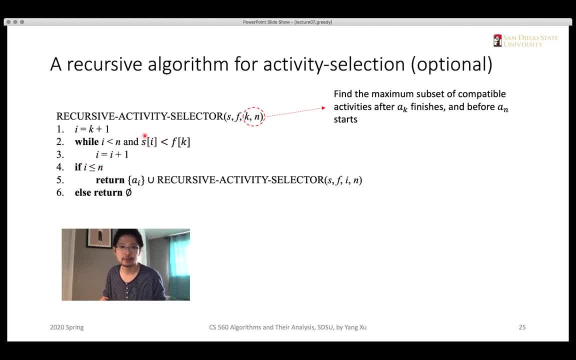 exceed N. it means it is this condition, the break of this condition, that terminates the while. so which means activity. I should be selected to be the next activity after a K and after AI is added into the final solution. it will recursive call in, invoke a recursive call to the algorithm itself, to the port, to the procedure itself. on the. 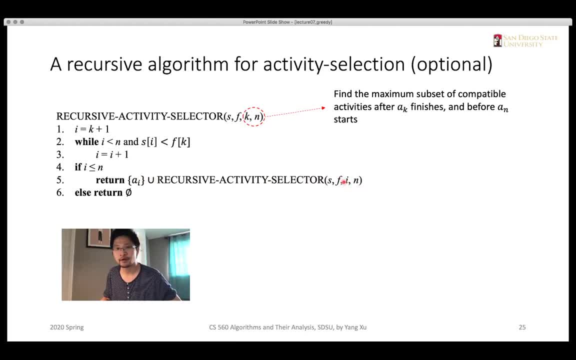 different sub problem that starts from activity I and ends with activity N. okay, so this is an example of a recursive call to the algorithm itself, to the procedure itself, on the different sub problem that starts from activity I and ends with activity N. okay, so this here, line 5, is where the recursive call happens. okay, so in order. 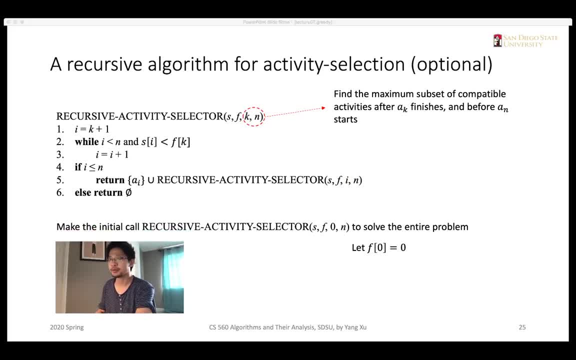 to solve the original problem that ranges from 0 to N. say, if you have N activities to select, you just need to invoke the initial call on 0 and N to solve the entire problem. and there's one more additional input is that the F of N, the F of 0, should be 0. so this is a special 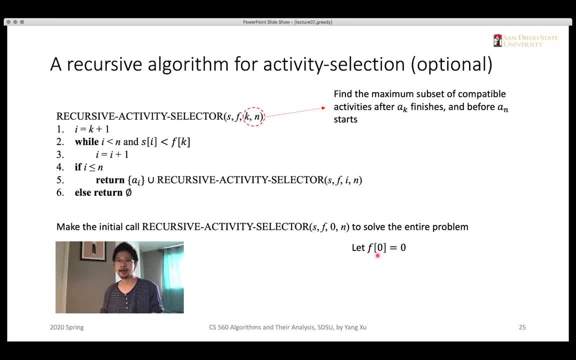 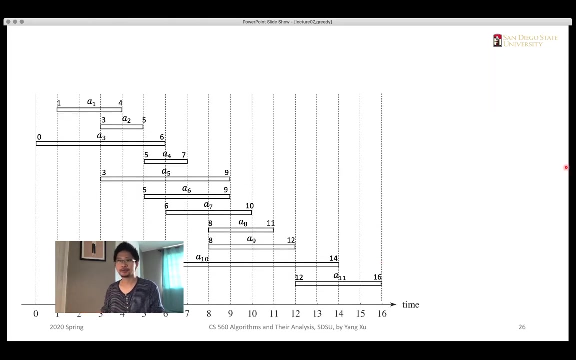 elements that will be needed, because in the original table F ranges from 1 to N, but here we will need to use the information F of N. well, when we call the, when we call the function initially. so in the next page we will see an example of how the algorithm runs on the inputs we have here. okay, 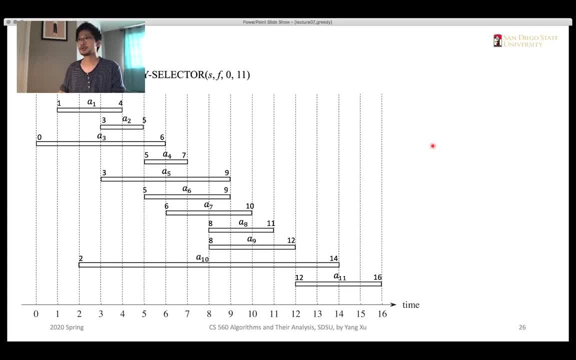 all right. so, in order to solve the problem, the original call should be recursive activity selector on 0 and 11. okay, because we have 11 activities in total. Okay, okay, so the while loop, the while the. i will start from one. okay, because initial k is zero and the while. 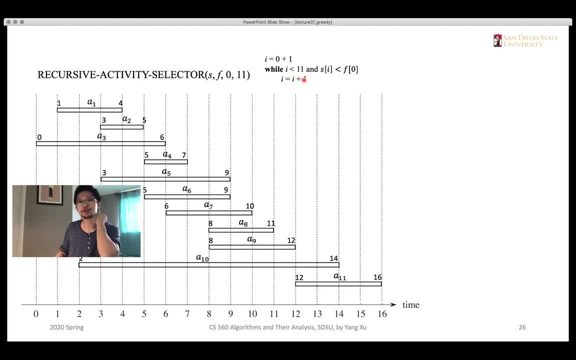 loop will increments i by one until either one of these two conditions breaks. okay, so when the while loop first breaks, the i should be one. okay, because the s1 is the smallest value, that's smaller than f0. we know that f0 is zero. okay, because k is. 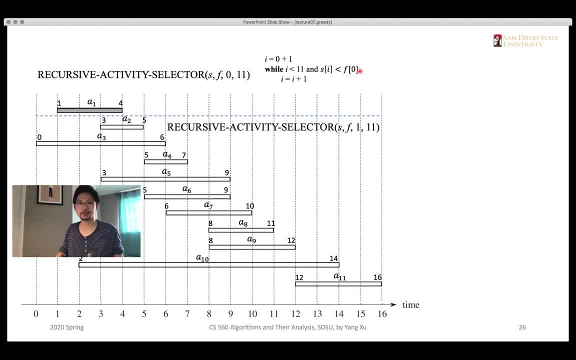 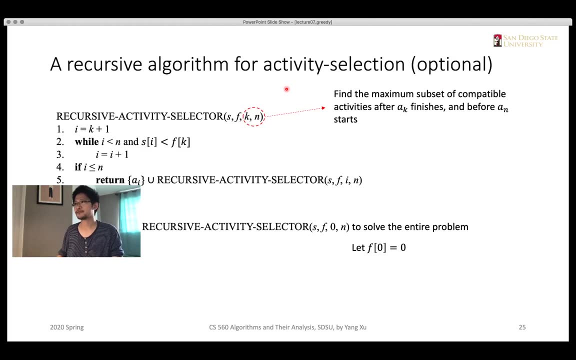 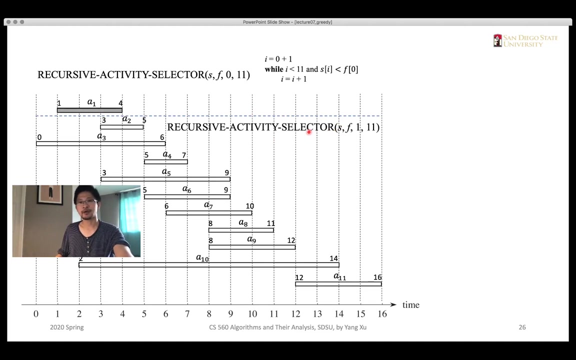 initially zero and we deliberately let f0 to be zero. okay, so that's how we select a1 and it will. after a1 is selected according to line five, we will initial we will invoke another call on: i equals one. okay, so this is a recursive call. so after a1 is initial, is selected, we will invoke the recursive call to the function itself. 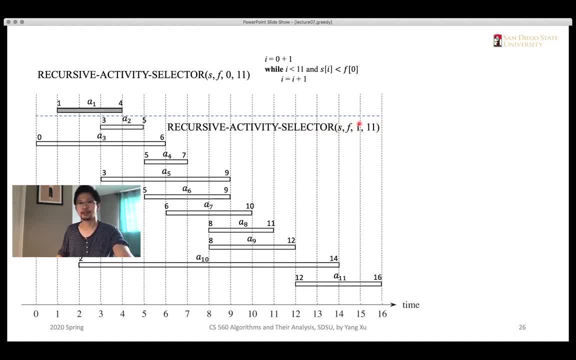 on one between one and eleven. so here k, uh, here one is the new k. okay, and within this call, i will start from two okay, and we will increment i until either one of these condition breaks. so when i breaks, i is four, when the while loop breaks, i is four. okay, so i four, eight, four is. 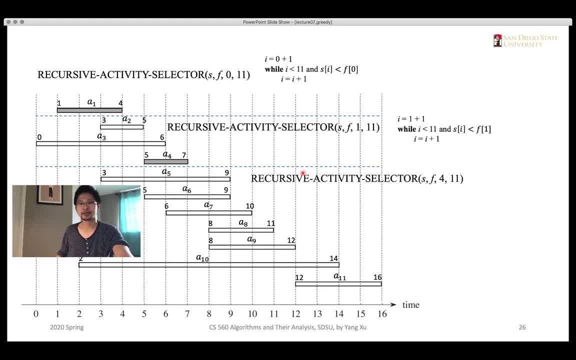 added to the final solution and the next recursive call will be between four and eleven, okay, and now, this time, the i will start from four plus one, okay, and the next one that satisfies is i. eight is eight, i equals eight, okay, and after a is uh, selected. 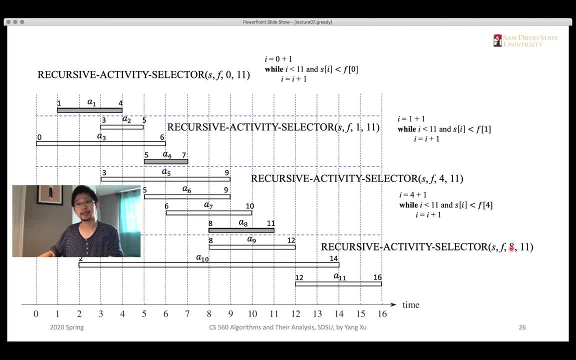 it will be added and the next call is from eight to eleven. and lastly, after a11 is selected, it will invoke another call, in which case, um, i will start. 11 plus one, okay, but this time the i is bigger than 11, then i the. the while loop will break and in the, in the next line of the if 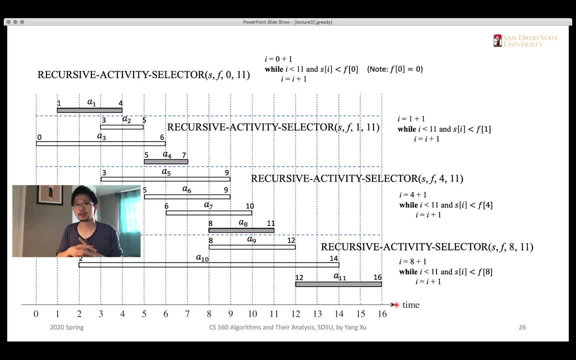 condition. it will check whether i is smaller or equal to n, and that is that if condition breaks, so um, there will be no more events added, no more activity added. okay, so that's how- a recursive activity, uh, recursive way of solving the activity selection problem using the. 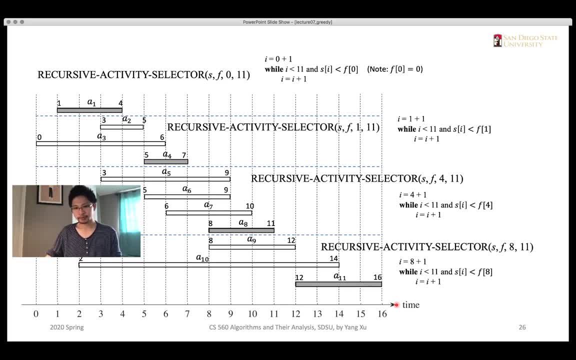 same um greedy uh strategy. okay, and uh. i think uh, this recursive way is not as easy to understand as the iterative way, but as we run through the examples, they are basically doing the same operations on the same inputs on the same input data. so that's it for the lecture today, and uh. 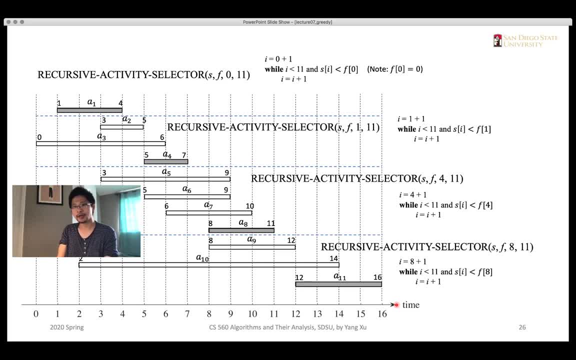 i hope you uh find this video useful and remember that there is a quiz um that you need to submit, so you need to write down the answers on the on your paper, on one paper, and then you take picture of it and upload the picture to the blackboard system. okay, so from next lecture on. 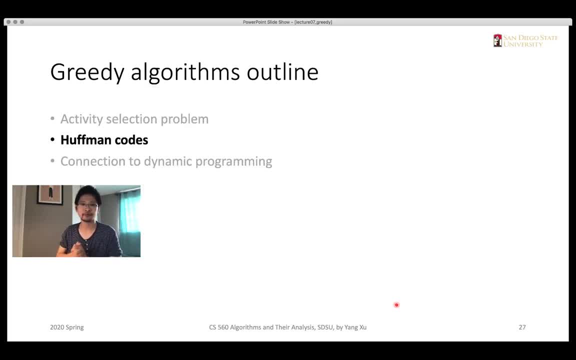 we will talk about halfman code as a second example of algorithm. the applications of 3d algorithms bye.